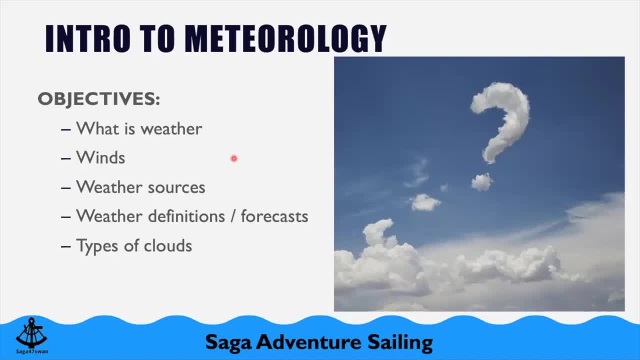 Weather definitions And type of clouds. Weather mythology is a massive, a very, very big topic, So it's impossible to cover that in just one session. So, as I mentioned earlier, it's huge. it's like an elephant, so we have to eat it bite by bite. 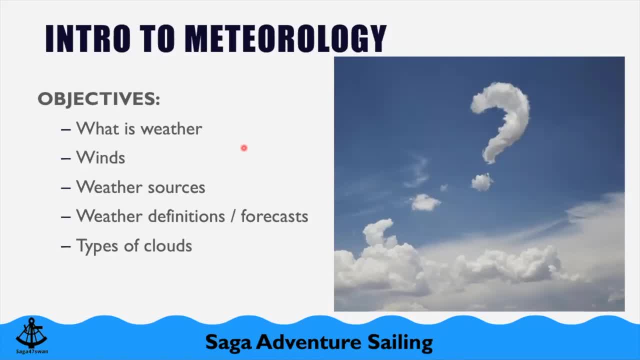 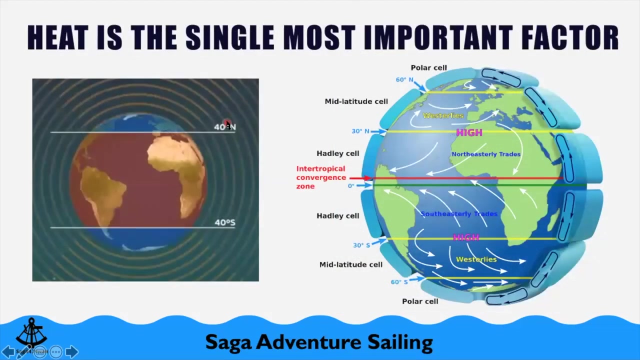 So this session is just the first step in that direction. Next week we will have a second session where we'll be looking at weather fronts and weather Pressure systems. Another poll, hang on. So what? what factor do you think is the, let's say, the single most important factor that drives our wet weather systems? So it is heat. Heat is the most important factor that drives our weather systems. 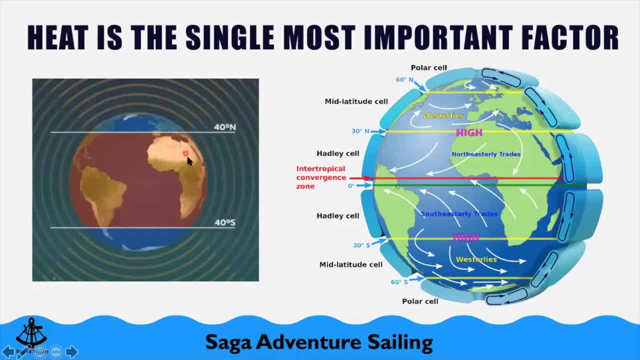 And, as you know, the earth is heated by the sun, so radiation from the sun And the sweep causes much heat, So most heat hits us at, hits the earth and the crater And then, as we move towards the polls, lesson this: he is a. 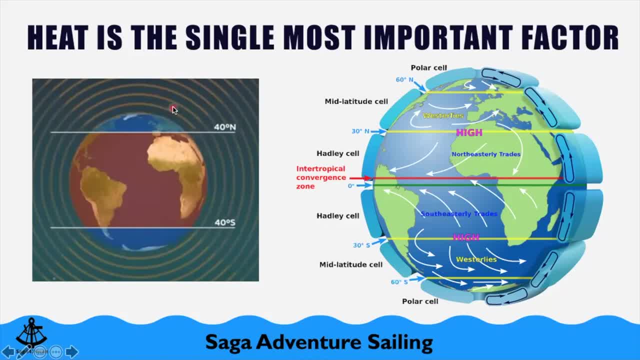 Is a transfer to the year to the earth. Actually, when we get to 40 degrees North or south, Then The amount of heat that is radiating away from the earth is more than what is coming in from the sun system. our weather system is actually like a big air condition unit that brings the heat from the 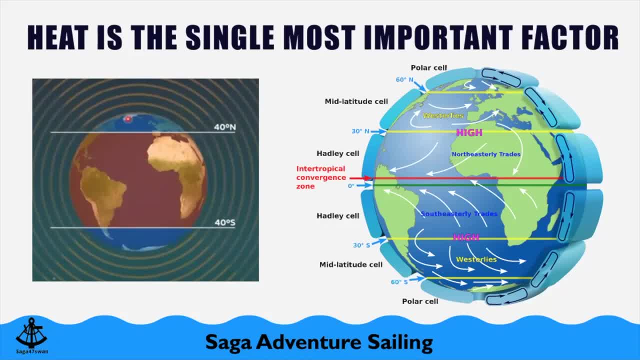 crater area up to the poles. if we didn't have our weather systems of winds and so on, then the poles, the two poles, would get so cold that nothing could live there and, of course, a crater will get so hot that nothing could live there. let's look at that in more details. so the four elements: 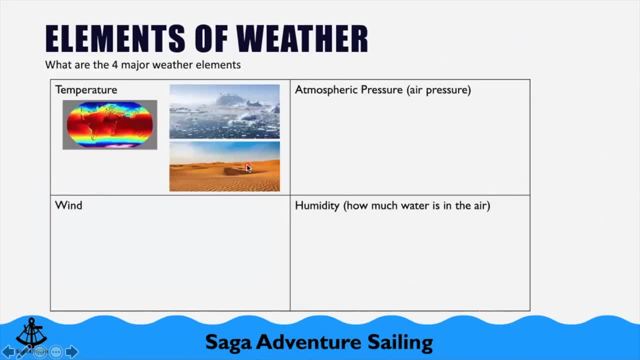 of uh, of weather elements are temperature, so temperature differences, that means hot, cold. we look at air pressures and so that means the gravity of the air and the uh, so the density of the air and the air pressure. we'll talk more about this in a bit. of course we have the winds, so the winds are blowing, winds are driving, also the weather. 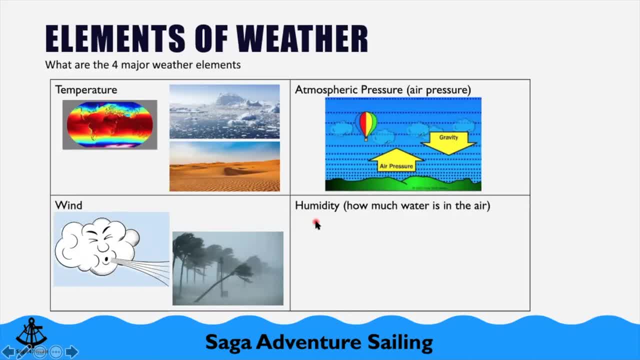 systems and the humidity. humidity of the of the air. that means how much water is in the like in your, in your bathroom. the hot air is there. when it cools down, it condenses. that's the same things we will see in the spring in the uk when hot, humid air is coming from the atlantic, south atlantic, into 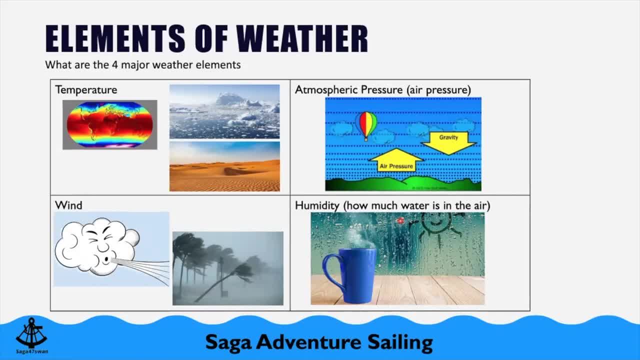 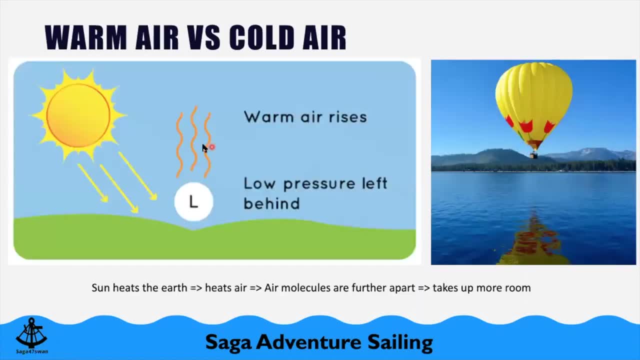 the cold waters of the uk, we get the fog. so same principle. so let's have a look at this in more details. what is driving this? so the sun heats up the earth and the earth is actually what's heating the air below, and when the air is being heated, it rises up, it gets, it gets hotter and it rises and the air. 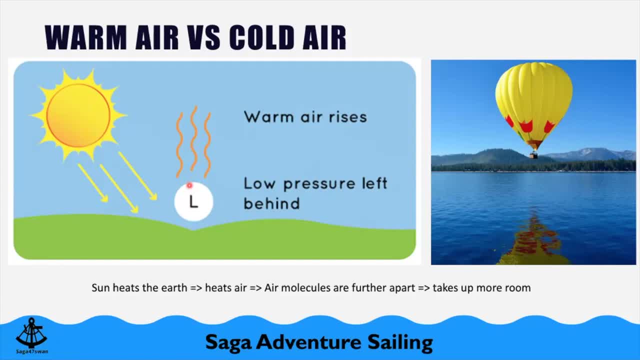 molecules, uh, gets further apart. that's the same principle as we have in a hot air balloon. when we heat the air in a hot air balloon, the air gets hotter and the air molecules gets further apart. it takes more air space and that makes the air balloon rise. 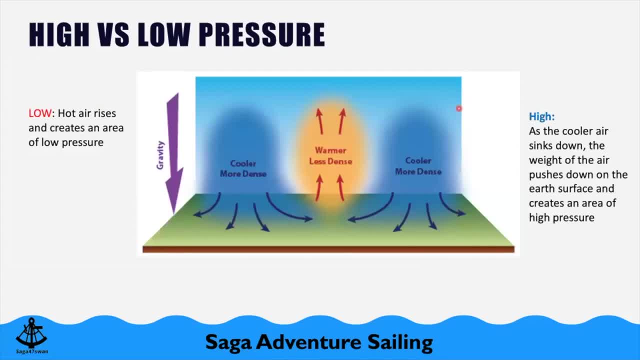 So that generates a high and low pressure system. So the hot air is rising up and when it comes up to the top it goes over and it starts to cool down and it starts to descend again, cooling down, becoming more dense, generating a higher pressure on the surface of the earth. 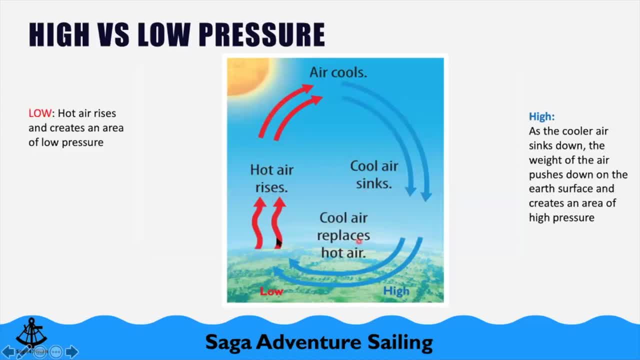 So that generates this cycle here. So hot air rises, it cools, it sinks down, it generates high pressure. The air that rises has to be replaced. so we have hot air going from high pressure, sorry, cold air going from high pressure towards. 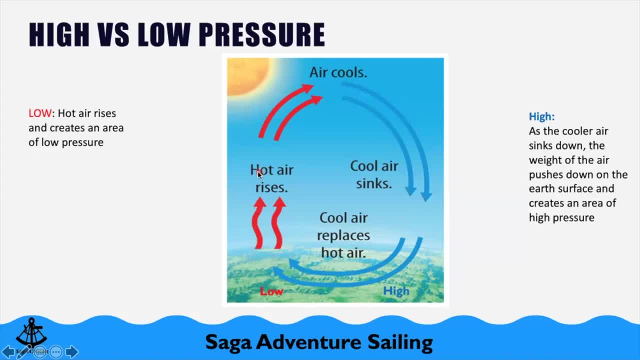 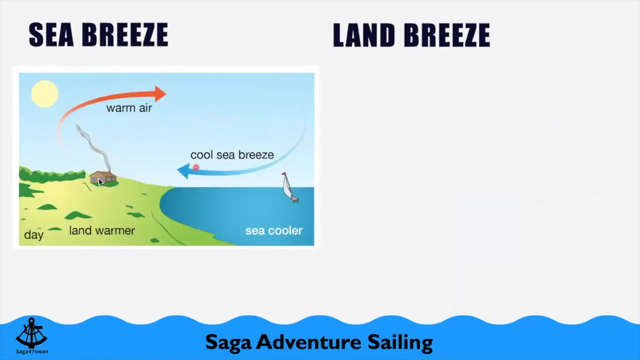 the low pressure and that generates this system. here It's like, because the furnace will be heated up, here it goes over, it drops down and generates this cycle. You probably experience this when you go to the beach in the summer, Because in the summer, when we are on the beach and the sun rises, the sun starts to heat the 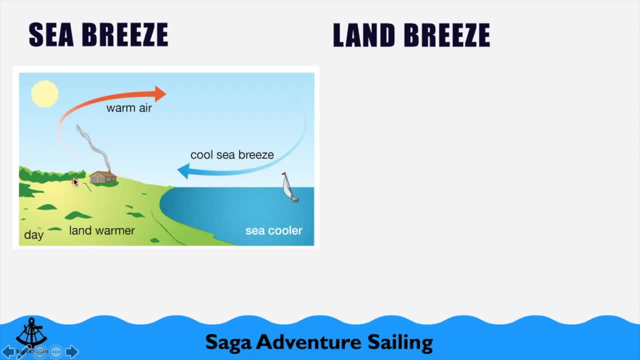 land and the air. land warms up and the air starts to rise, goes up, it moves out towards the sea. the sea is cooler, drops down and then starts this cycle. A lot of people they go, for example, in the Met. 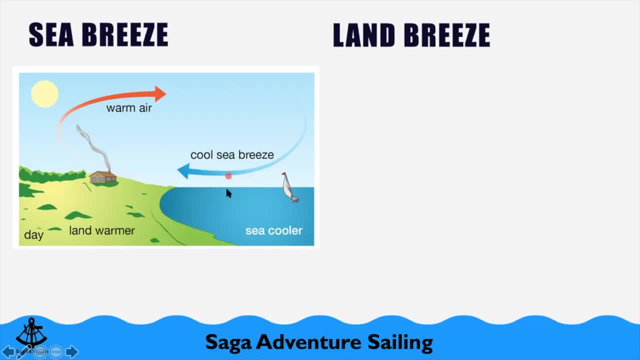 so they go to the beach or they have their boat, they sail in here. they arrive here around lunchtime. ice force 2, force 3,- lovely, they get the picnic out, the white wine, and then suddenly after lunch we get a force 5 and that is the sea breeze. that is. 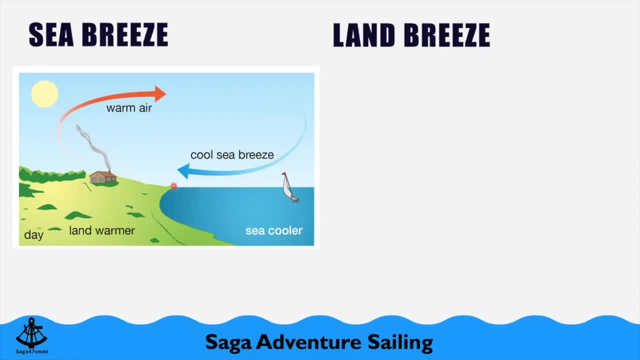 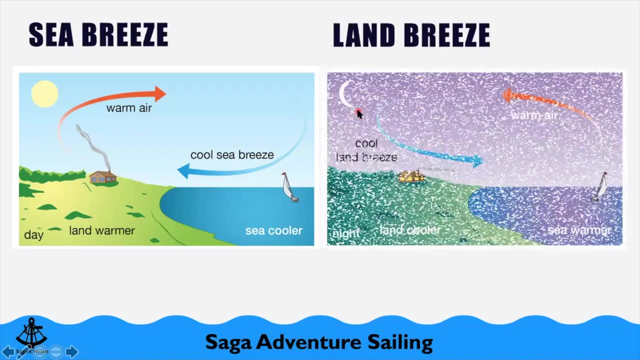 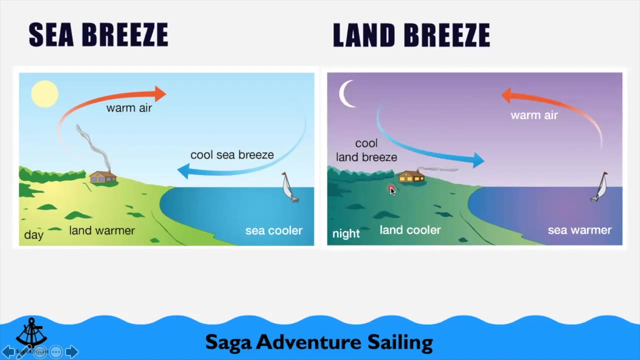 blowing in. It's very, very. they can be very, very strong in the Met, but of course also here at the south coast in the UK. In the evening we get the same system. the sun goes down. the land will cool down faster than the sea. that means the hot air over the sea will rise up, move in. 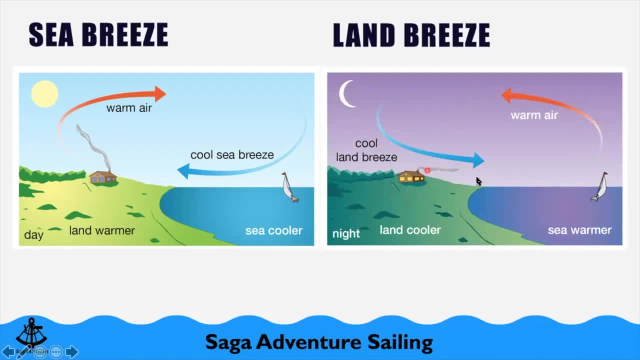 it has to be replaced. and then the cold air comes out. when we get this land breeze in the evening, in the night, Let's just bring up the pressure system so air will move from high pressure towards a low pressure. So that's the system, so that's the cycle there. Let's look at a bit more global. 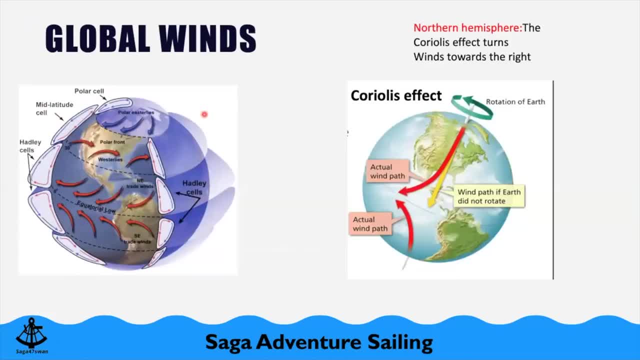 aspect. So we have global winds and this is where we bring in the Coriolis effect. So at equator it's very hot, so the air is heated up, it goes up and it goes towards the north or towards the south, both direction. it cools down, it drops down and 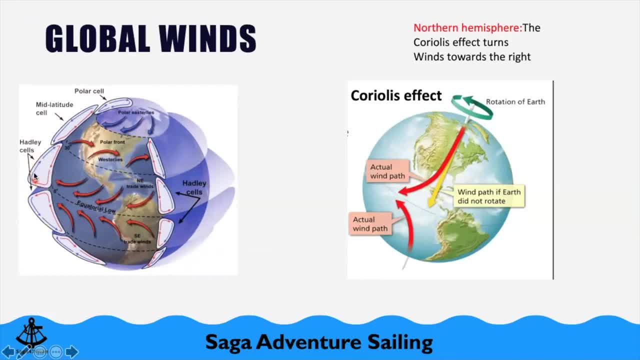 we get the Hadley cells, so they rotate like this The same thing we have up at the polar cell again. it's cold here and it's hot here, so they start also to heat up and get rotation there and the mid cells are driven like a wheel in a gearbox. so this one is rotating here and the mid 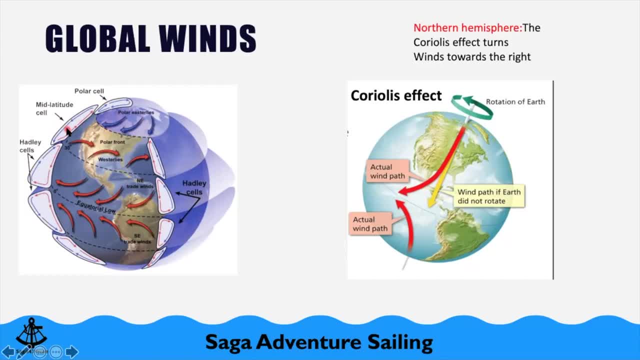 cells are rotating the other direction, But due to the Coriolis effect that means the earth is rotating. then the wind is not moving directly from north to south and it's sort of deflected and it turns in the northern hibiscus, it turns to the right and that's what drives our 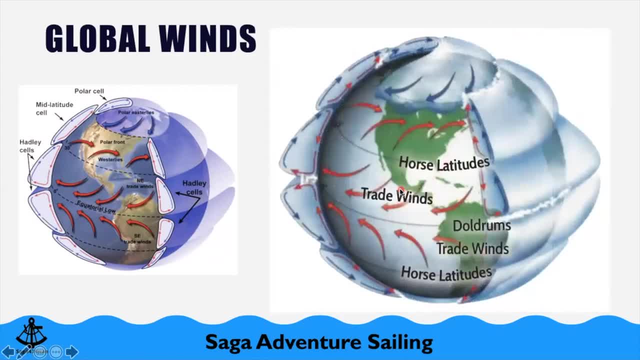 weather system and that's what gives us, for example, the trade winds found by the crater that we use to sail across the Atlantic and the Pacific in the in the in January. and well, December and January they're fully established in the in in January. We have something here called the 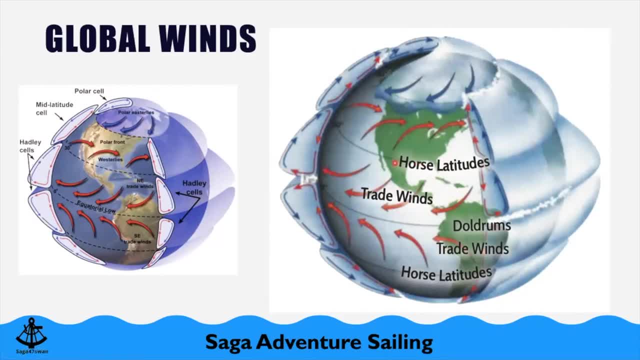 horse land. In the past they didn't have water makers also, and horses, they drink a lot of water. they could get stuck there in the in in very light winds. so in order to preserve water, they have to get rid of the horses, and they will throw the horses over the side. So that is correct. yes. 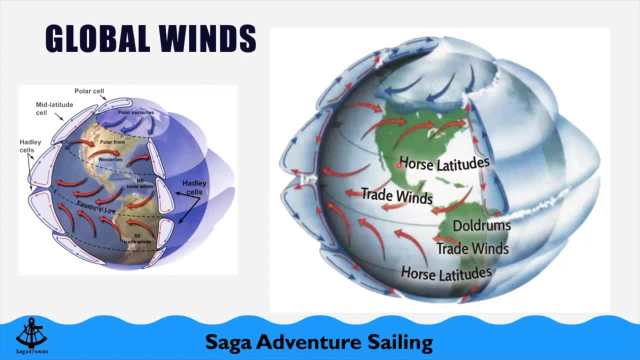 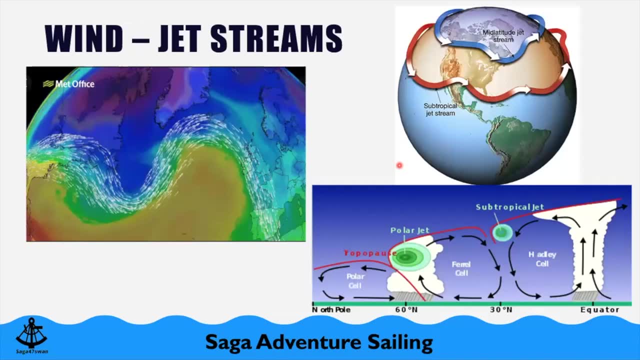 that's why it's called horse land too. Okay, we have also something called the, the jet streams. they're a bit high up and they are basically super conveyors, very high speed conveyors of winds, more than 200 miles. We have what is called the subtropical jet goes here, and then we have 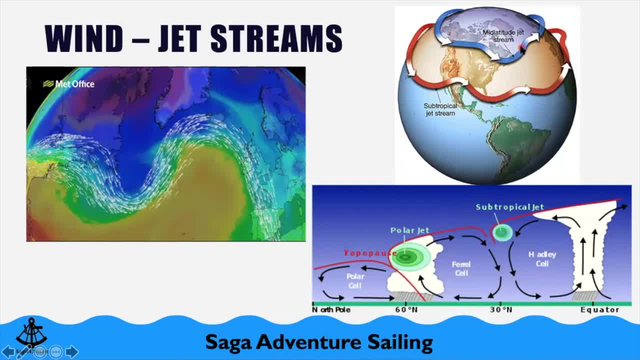 something called the polar jet a bit further up, and these are the ones that are driving our, our weather systems. yeah, They don't go. they go more like a snake. and the reason why they go like a snake is because, as they go over land or sea, then the different temperatures and different 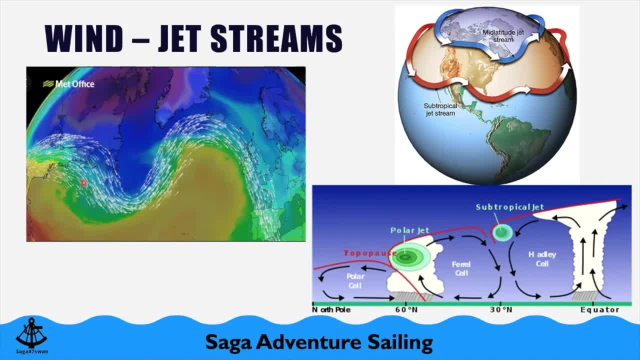 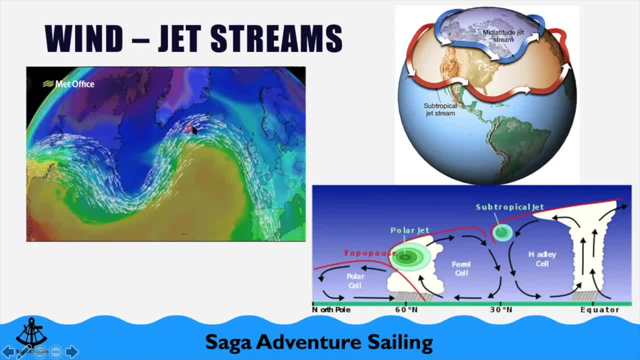 and that is what drives the, the weather systems, the depressions, that comes into towards the, towards the UK. Yes, there's some really interesting videos on the Met Office YouTube channel on on this, on these jet streams. Very, very well done and I highly recommend if you are more interested. 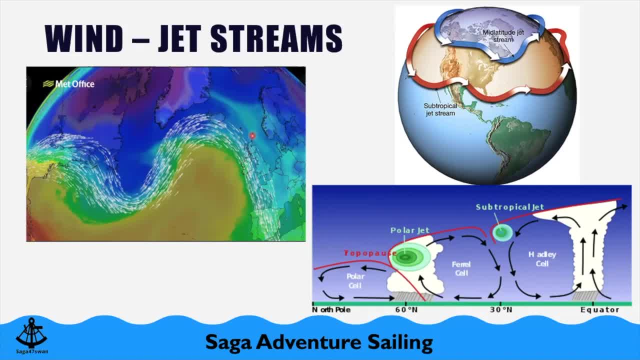 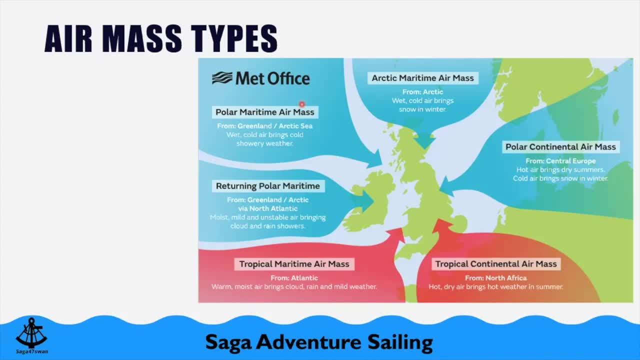 in learning about these jet streams, then it's really good to watch those. In order to understand also weather, we need to understand air masses, and there's different types of air masses. We have something called continental air masses and maritime air masses. So continental is coming from land, maritime will be coming from seaside. 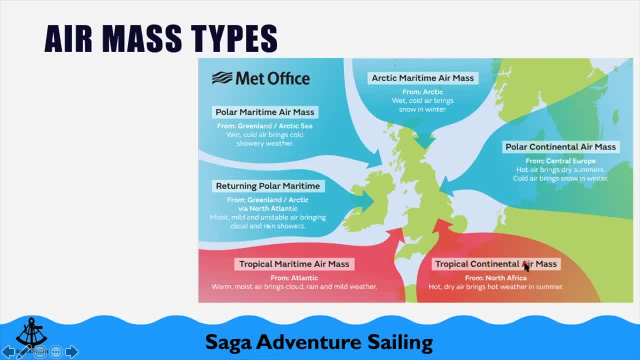 So tropical continental air mass is coming, for example, from North Africa. It will be dry because it's coming from land, and it will be hot and that can give us a very nice weather up in the up in the UK in the summer: hot and dry weather, Even though it. 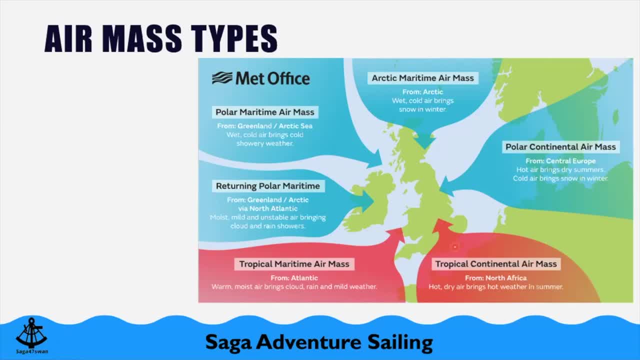 goes over the, the Met. it doesn't pick up too much water, so normally it will give us a very nice weather. We have another one, which is the polar continental air mass. It's coming from the, from the North Pole, and it goes over Russia and Central Europe. It's the. 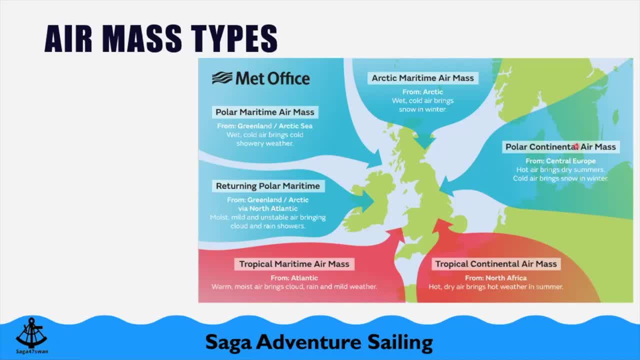 in the summer it can bring hot weather, but in the winter it normally brings very cold air, the beast from the east. It also picks up a bit of moisture from the Baltic and from the North Sea, so it can also give us a bit of snow in the winter. 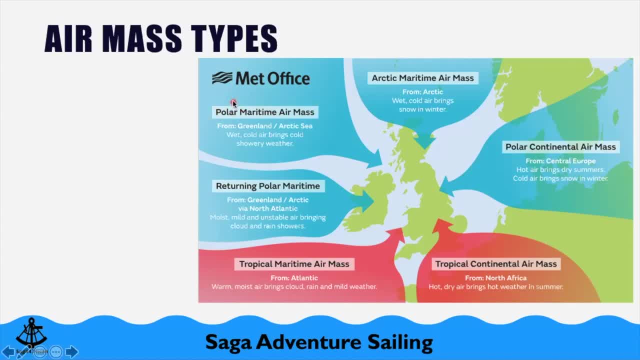 On the other side. here we have the polar air masses coming up from Greenland. They are also very. they start out very dry and then, as they go over the North Atlantic, they pick up a lot of moisture and then they will be bringing in rainy weather or, in the winter, and bring snow. 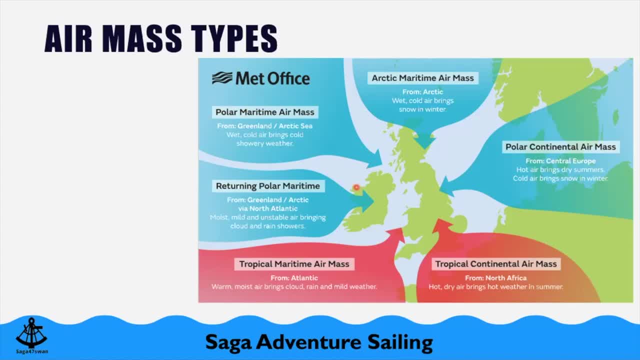 to the to the UK. The last one we have down here is the tropical maritime air mass. It comes from the South Atlantic and it's not going to be a lot of moisture, It's going to be very, very dry. So we're 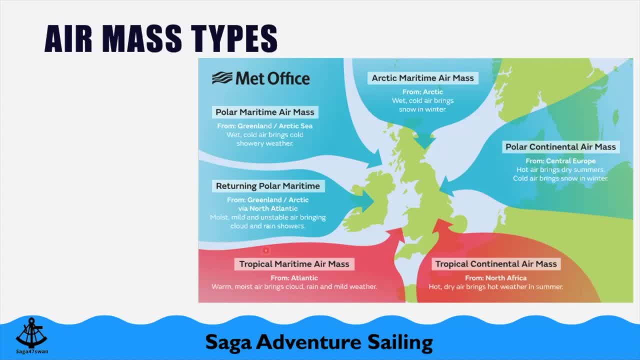 normally very warm and also very moist, And that is what can bring in the springtime. it can bring a lot of fog to the UK, So we get the sea fog down in the English Channel a bit like your bathroom again: hot, moist air, and then it gets cold and it. 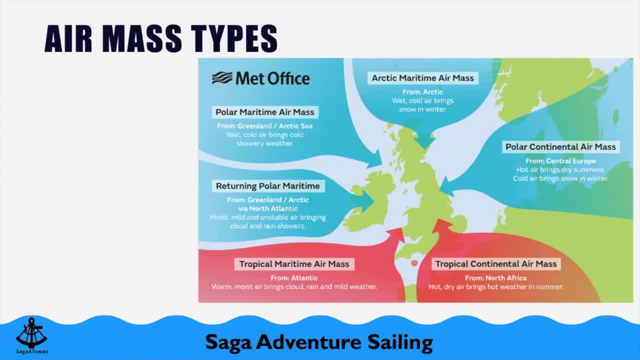 condenses and gets sea fog and you can have that fog lying there for several days. So that's why if you are sailing in the UK in the early spring, then it's very good to have, like, for example, a raid on your boat or stay in port when the fog is. 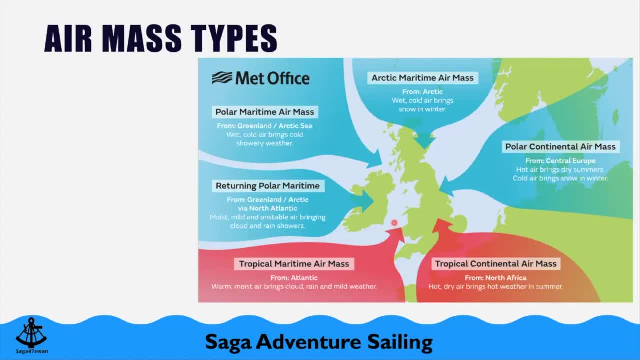 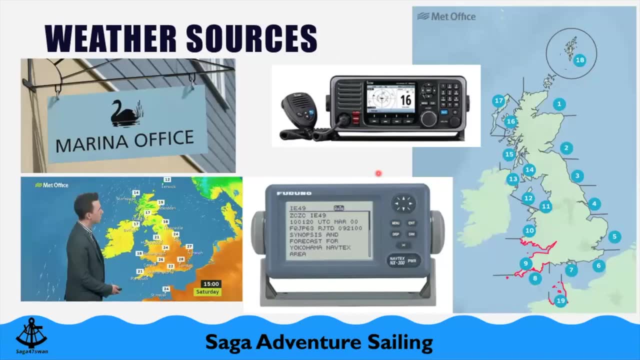 out. Yeah, okay, Now where do we get information for about the weather forecast? we can get information on the weather forecasts from, for example, television or radio Or a lot of people the neglect that, but marina office, if in the marina you can, they. 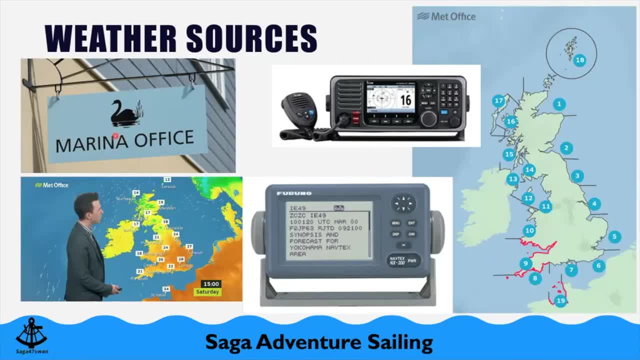 most likely have a. they would have a notice board or they even have maybe a computer showing the weather forecast. If we are at sea, we can get the weather forecast from our VHF radio, Or we can also get it from the nap tech system Or, finally, we can. 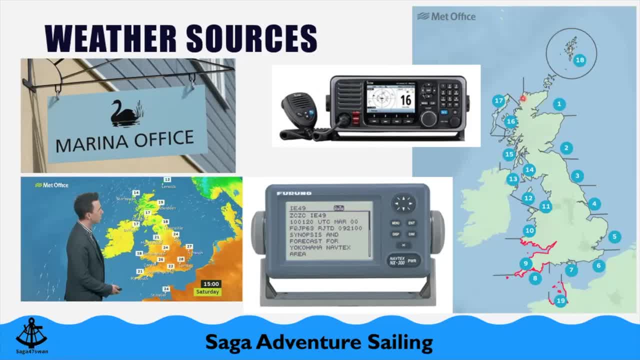 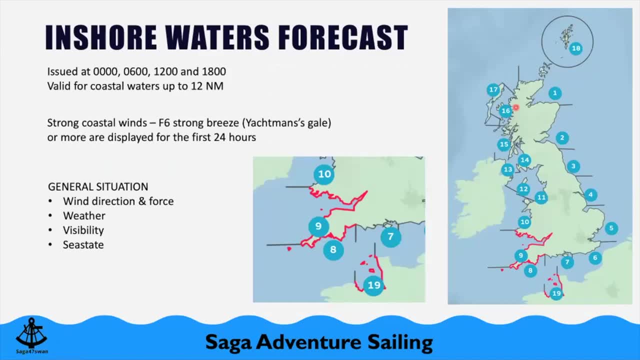 of course, get it from the, from the internet. Let's look a little bit more about. the one that we use mostly in the UK is the inshore weather forecast. It is issued four times a day And it's valid for valid for the coastal waters up. 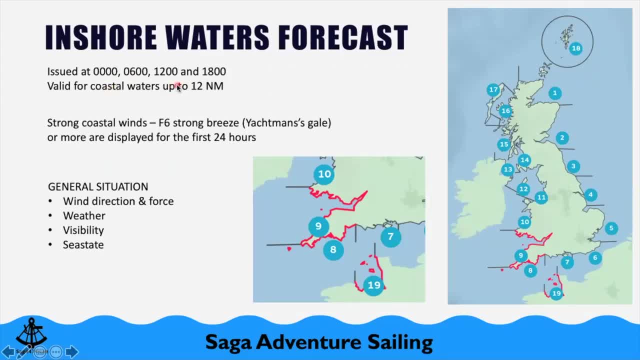 to 12 nautical miles from the coast. It has strong wind warnings. That means when the wind is f6, you call it yaksman gale- then the coastline turns red. So we know that there's a strong wind warning. 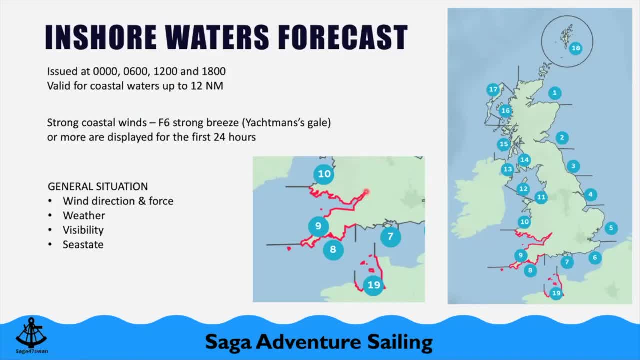 It gives us information. we look at it in more details later. it gives us information about the general situation. it will talk about, for example, higher low pressure, and then it talks about the wind direction and wind force, the weather, rain or 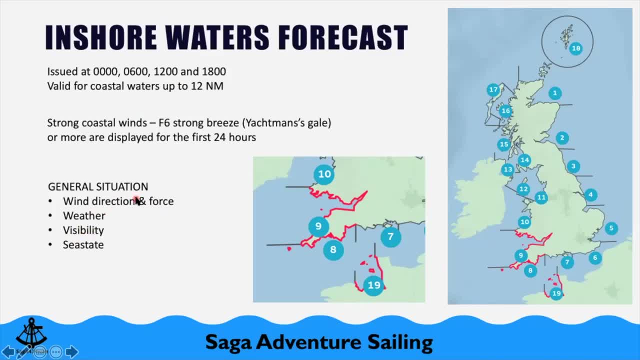 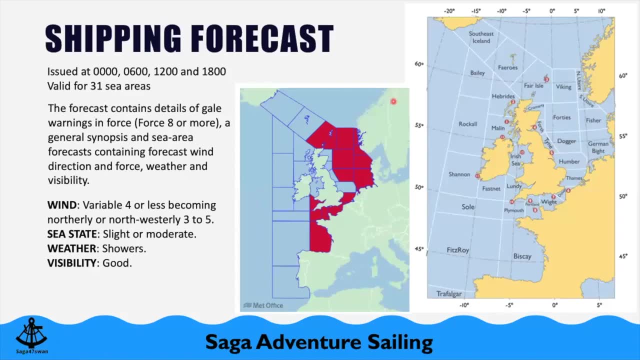 snow visibility and the sea state. If we are going a bit more offshore, then we look at the shipping forecast. So the sea areas around Britain is divided into 31 areas. Again, the shipping forecast is issued four times a day And it contains information, again about the wind. 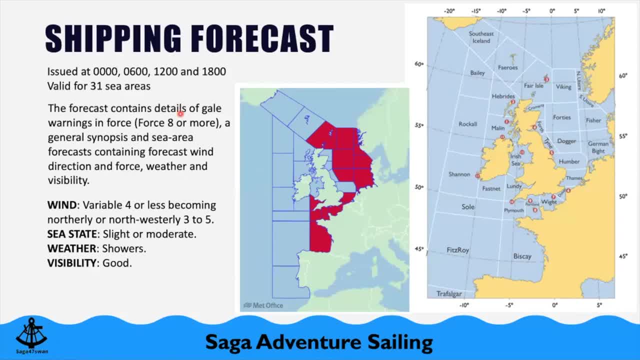 sea state visibility and so on. What is important is, if there's a gale warning, that means force eight or more, than the areas as you can see here will turn red. If you are planning to go sailing offshore, for example, if you want to go across the channel down here and 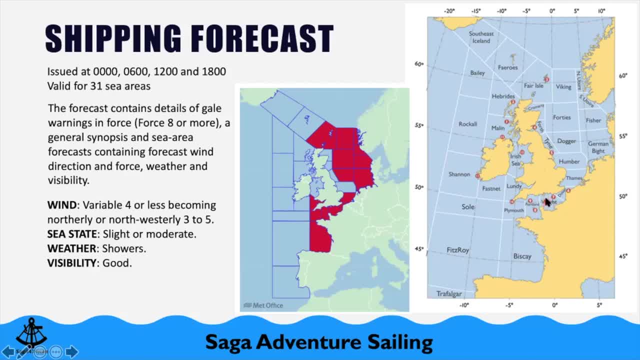 then you go from Isle of Wight to Sherbrooke, you will be in the sea area which is called Wight. It's always good to check out what's happening in the sea areas which align to the west of where you're going, Because what is the sea the weather systems will move from? 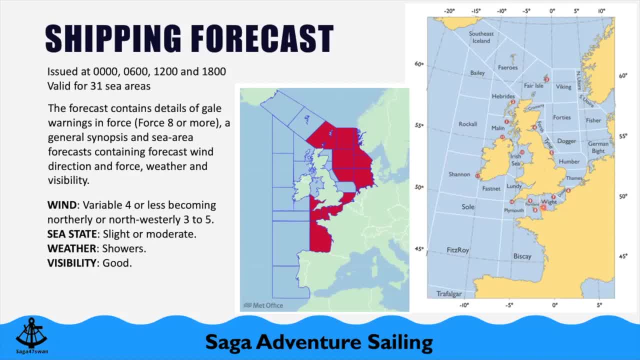 west towards east. So if you are sailing down in this area here around Plymouth, or you want to go to the land's end, Falmouth, or so on, then you will be looking at Seoul and Fastnet to see what's happening there, because that 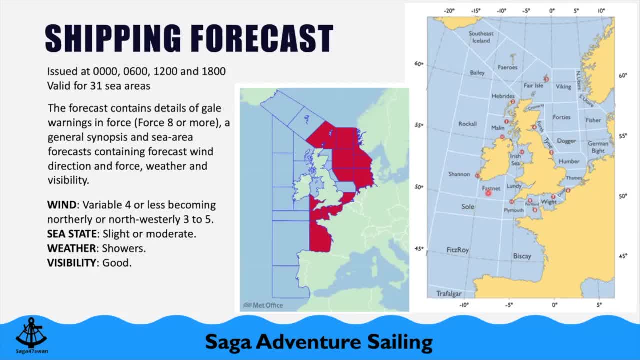 weather system is going to move towards you. So if you, if you look at that system, you will get a good idea of what's coming for you. You're sailing off offshore. you're not sailing just for a few hours, you might be sailing overnight or several. 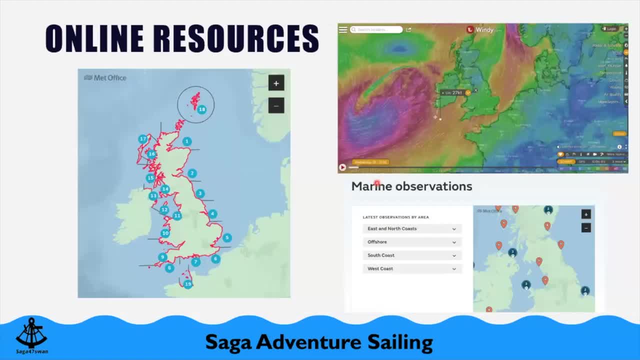 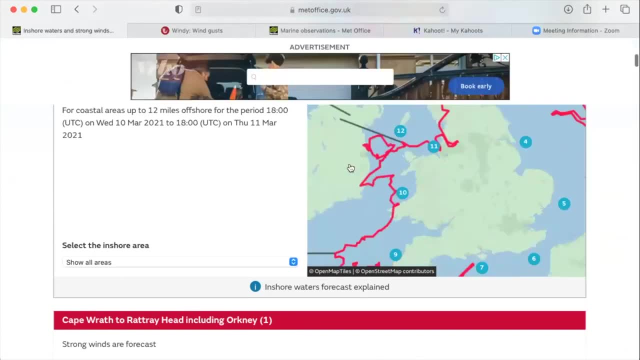 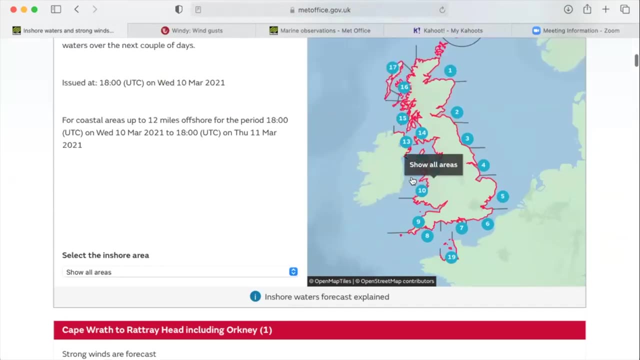 days Online resources. this is the inshore weather forecast. As you can see- we also talked about that earlier- All red all around it. That means the strong wind warnings for all areas, all 19 areas. This one here is issued just at the six o'clock, So 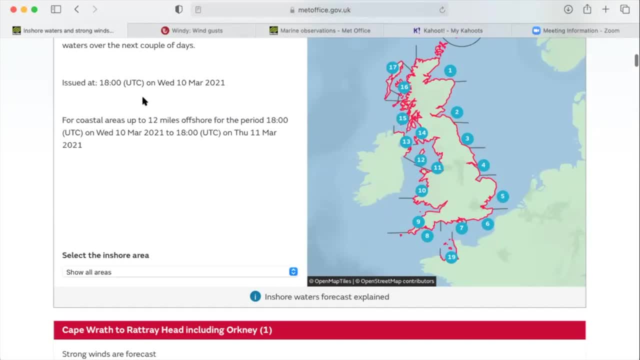 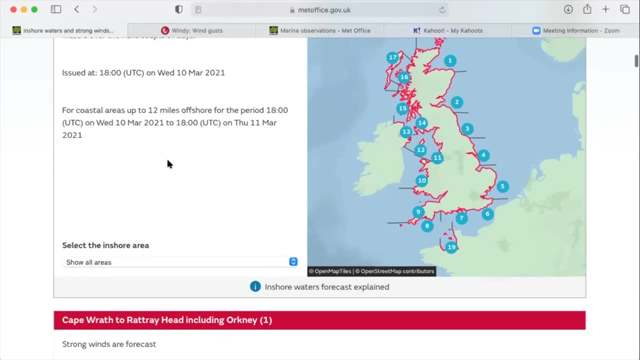 that's one and a half hours old. So you have to be careful when you're looking at weather forecast, because it's not at the time when you're looking at them which they are valid for their valid for the time issued. So let's bring up, let's look at. 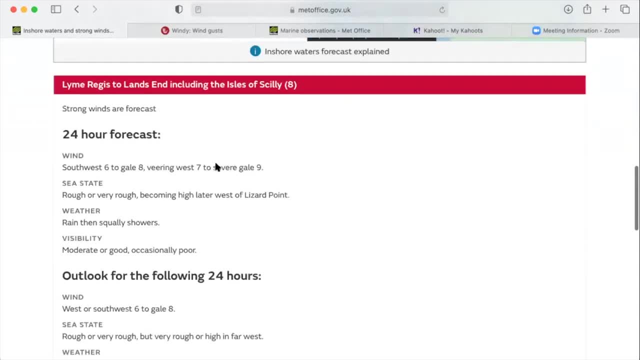 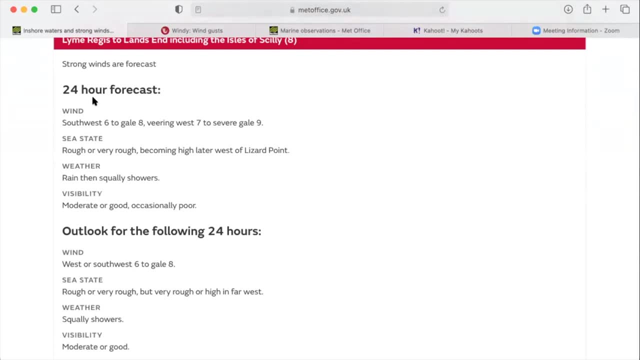 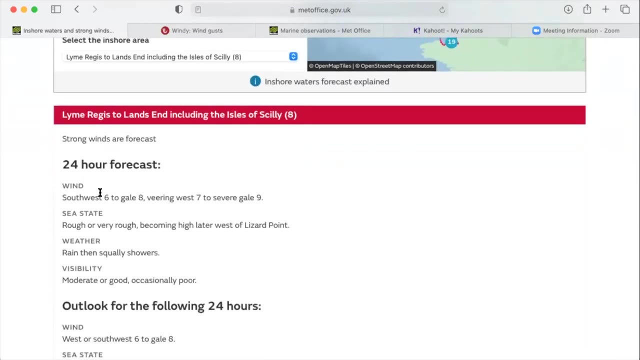 Plymouth Down here. So Plymouth. so this is the 24 hours forecast. So that is valid from six o'clock this evening until this is 24 hours, but the forecast is valid for the next six hours. That that gets very important when you start looking. 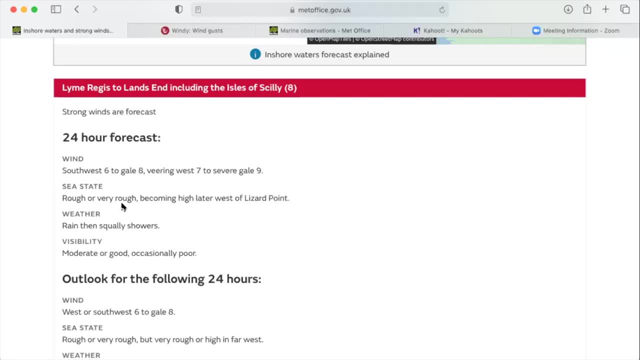 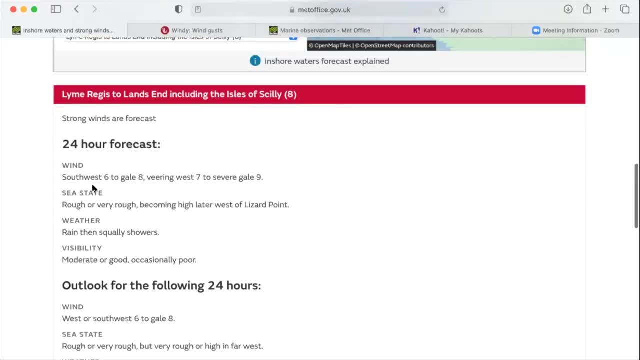 at what is happening down here, if it's turning later or imminent gale forcing, imminent, So one, But as you can see, it's quite, quite windy. It's going to get gale force nine. And very important is also to look at the 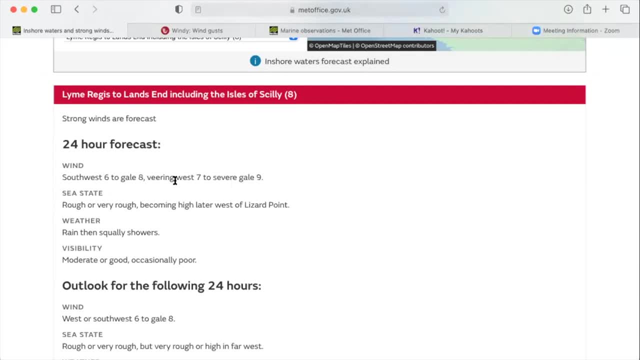 sea state, because the winds we can, we can. we can deal with the winds, so to speak, but we can make our sails smaller. But what is making the ride uncomfortable is the sea states. always very important to look at what's happening with the, with the sea. 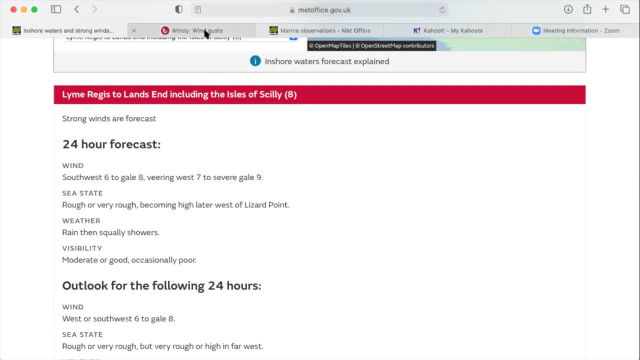 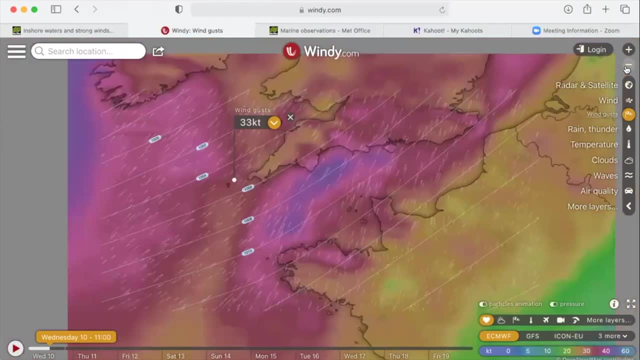 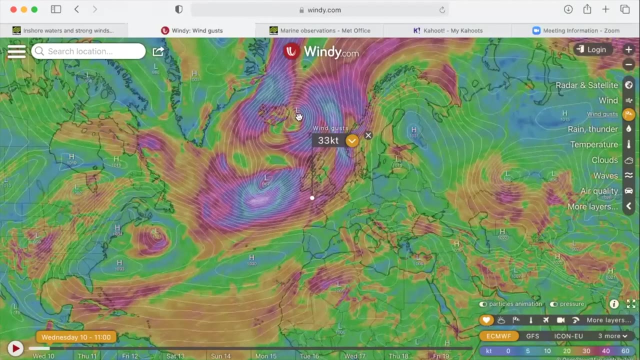 state with the waves. Another app that I like is windy. This is the window app. Yeah, you can look at the whole whole world. for that, Very good. Yeah, you can also see the reason why we're going. where we are having such bad weather. windy weather is these two low? 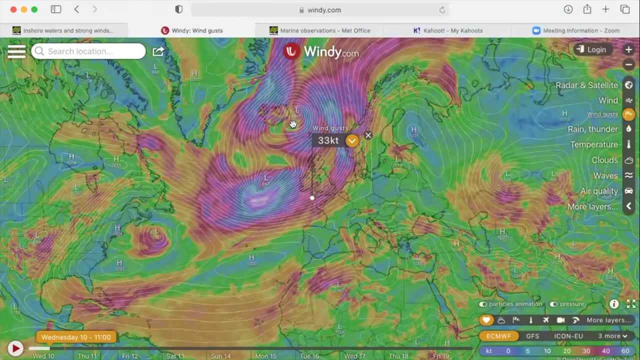 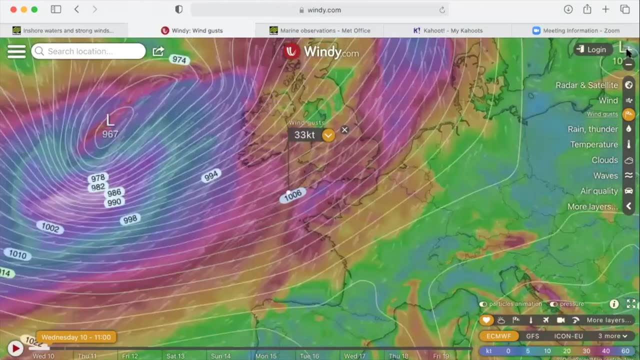 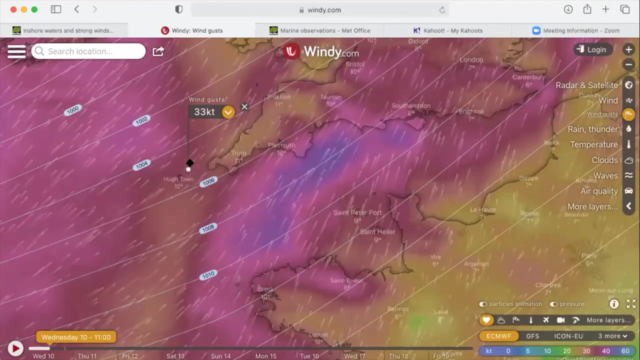 pressures here, very, very unstable systems at the moment of strong winds here And then when we see. So with the, with the windy app, you can also. you can look at different areas and you can get, for example, more information. So if I select an area down here by 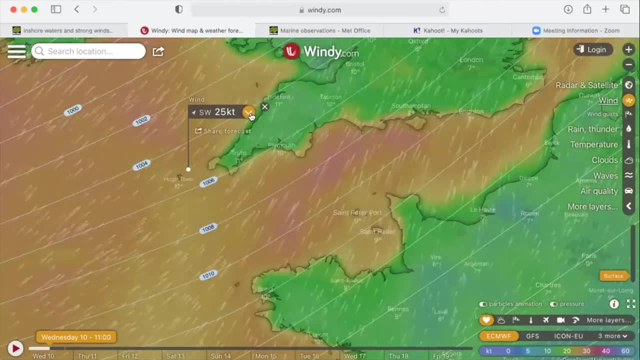 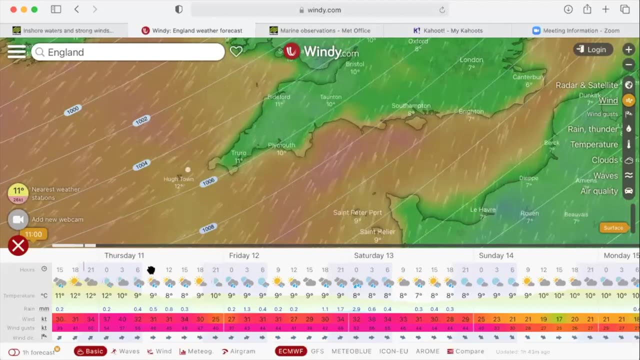 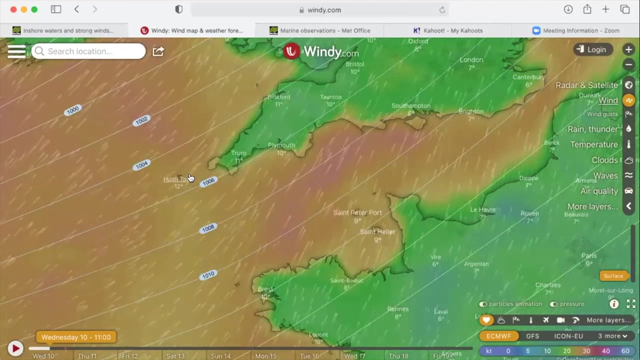 by the silly islands and then I can click on this one. I can get more information on that area. what's happening As we, as we progress towards the next days. You have to be careful when you're using apps like windy, because all these apps, there's many different. 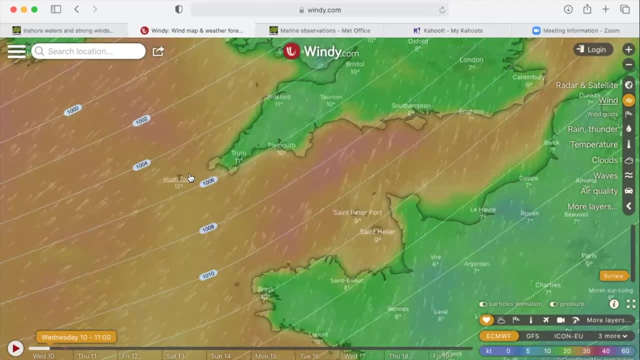 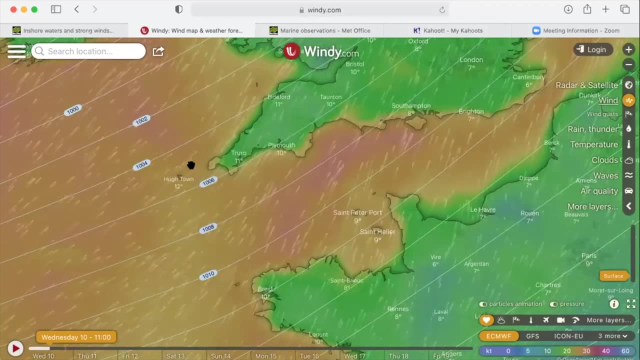 apps, but they're all based on the same mathematical models. Yeah, When you find an app that you like- I like some windy- then you can start looking at what's what's happening in real life And the way we can look at. 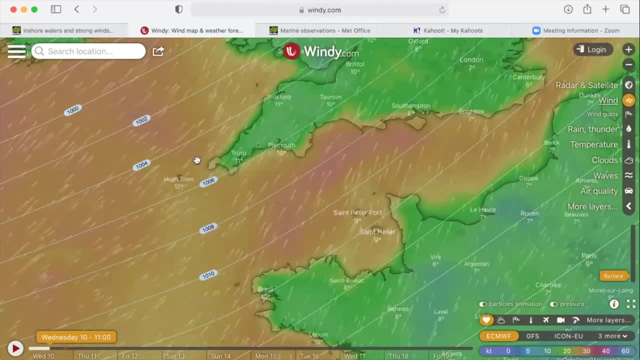 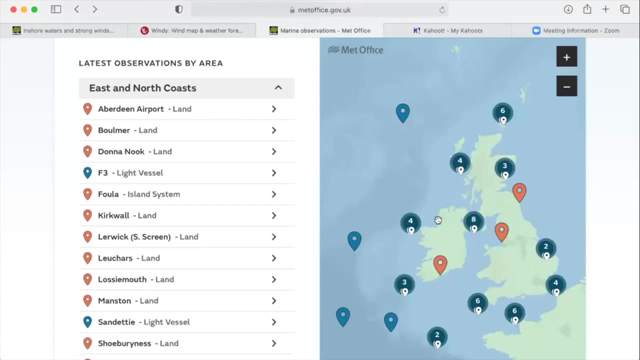 what's happening in real life is we can go into the middle of us again And we can say, Okay, here we have a boys out in the sea and we can look at those boys and see what is the actual what's actually happening. So let's see if you can find one. 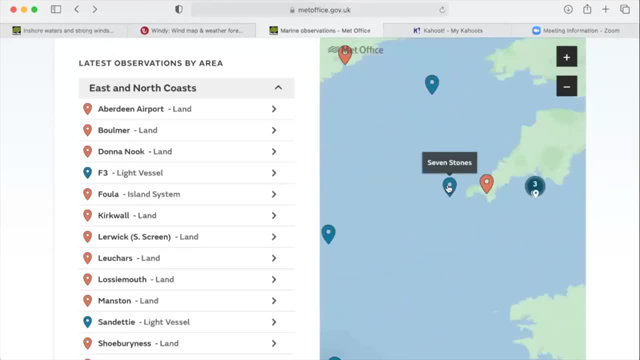 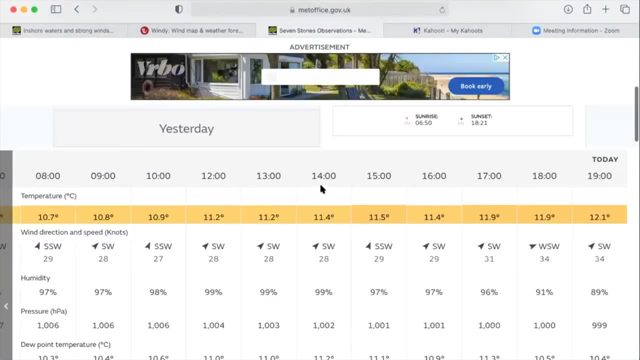 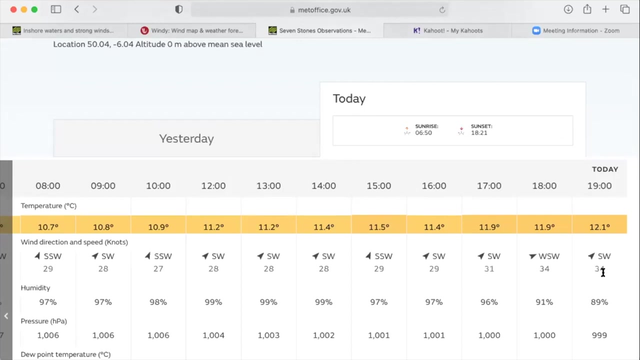 down by the silly islands, seven stones and click on seven stones, And then we say, Okay, what is so? we have here the historical data. And then we have, at seven o'clock today, just half an hour ago, southwesterly wind, 34 knots of of. 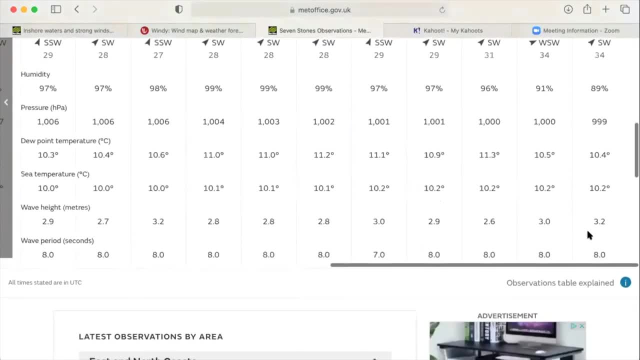 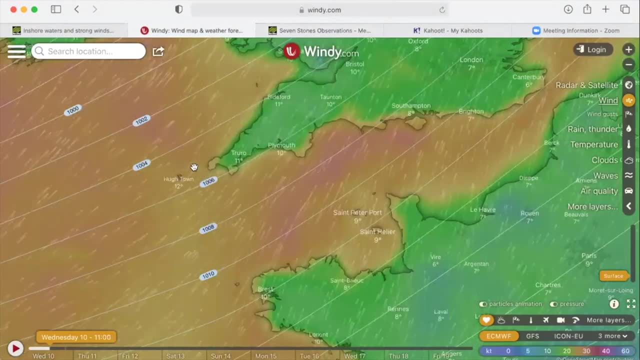 wind, And then let's go down and see what the waves are going to. waves are, the wave height is 3.2 meters. So let's go back to windy and then have a look. So down here somewhere. So there, Okay. 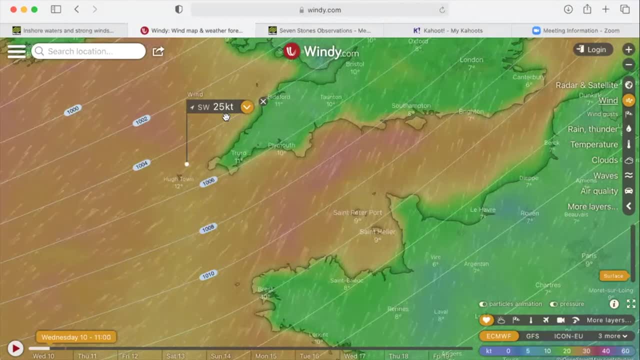 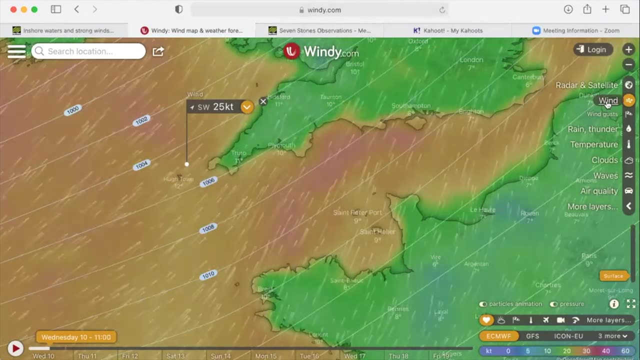 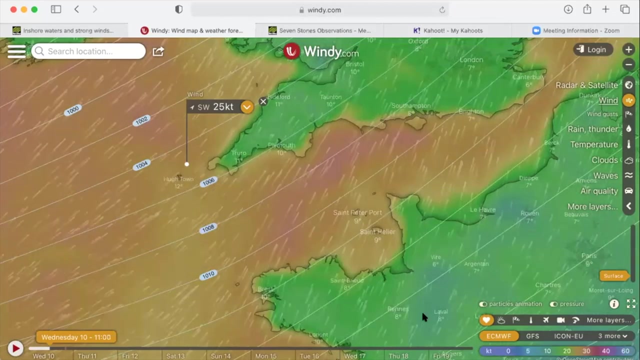 so says 25 knots. we had 34 knots actual down at the weather station. Yeah, And I also find with windy that if you use the setting which is wind- let me just get my wind gusts So you can see what I'm doing. So over here you. 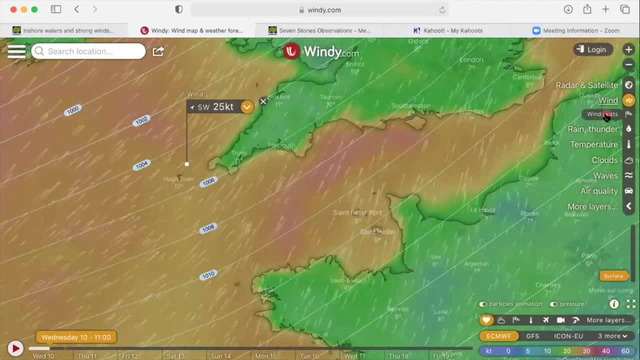 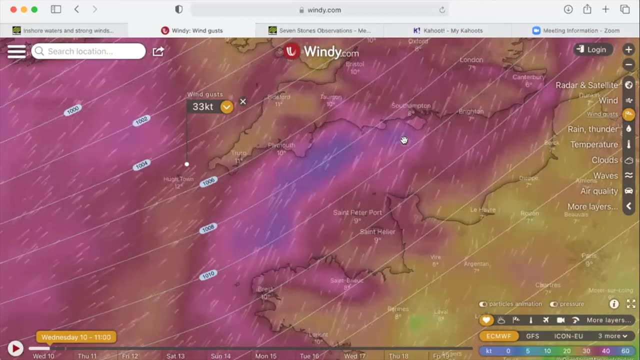 have the settings So we have something called wind gusts. So I find when I use windy it gets more accurate information on what's happening. If you use the wind gust setting, you can see now the wind turned purple. that means more wind And also we. 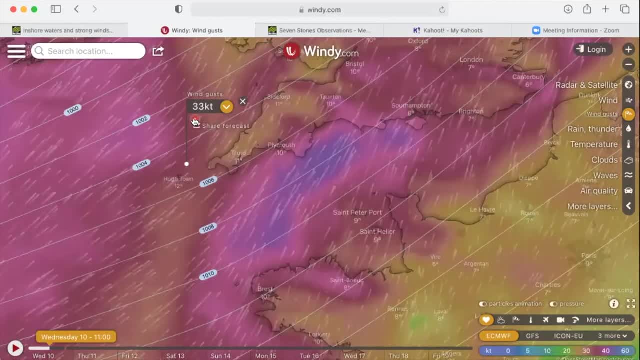 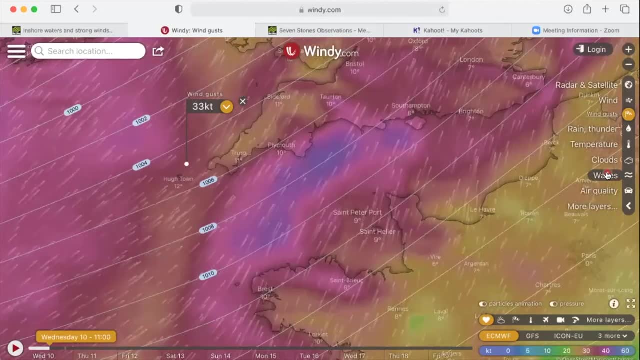 have 33 knots with. tell us more with what's happening down at the boy Windy can also give us information about the waves. There's a setting here for waves so we can check on the waves. So 3.5 meters waves, we had 3.4 at. 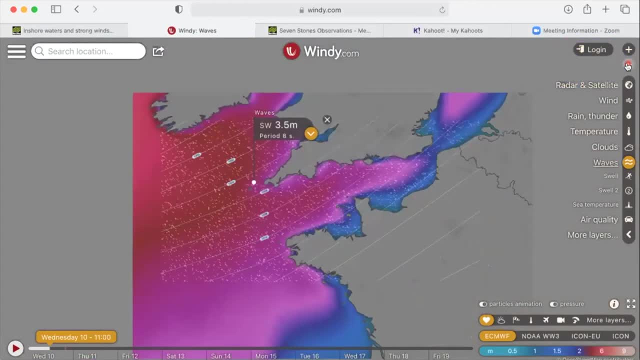 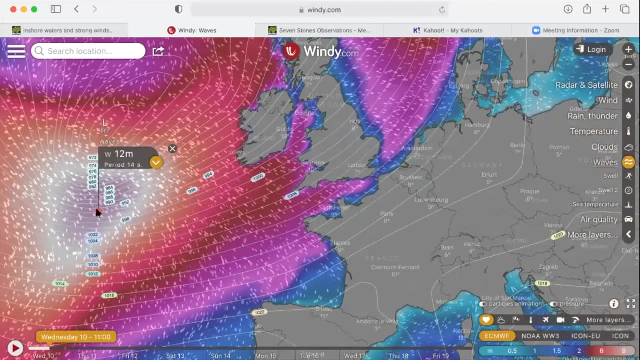 the boy. So that also tell us. very well, You can look what's happening out in the Atlantic. I think there's more than 10 meters waves out there, So we don't want to be out here. We have 12 meter waves out there, So that will not be very nice to. 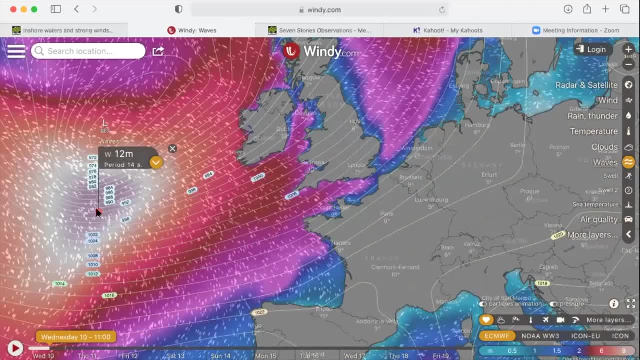 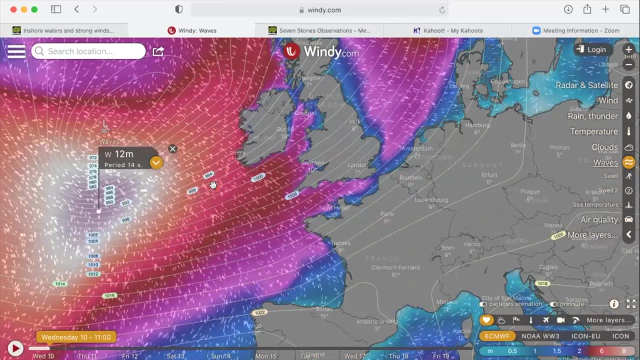 be out there in a, in a vessel there. So there's lots and lots of apps and you need to find the one that you're comfortable with And then check the weather and check what's actually happening when you're out sailing. So you know. 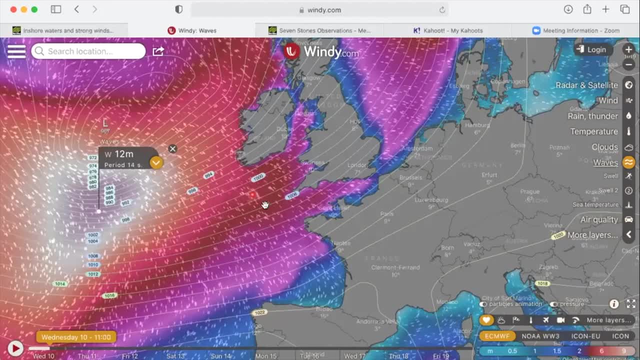 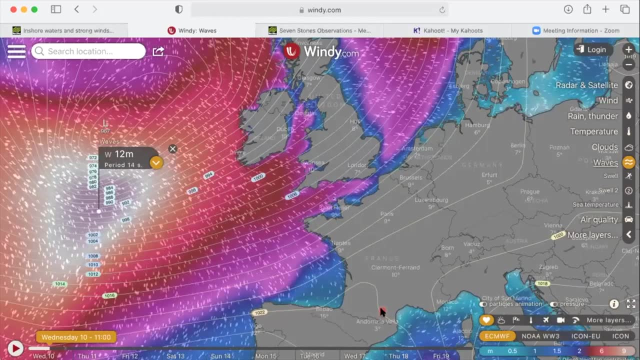 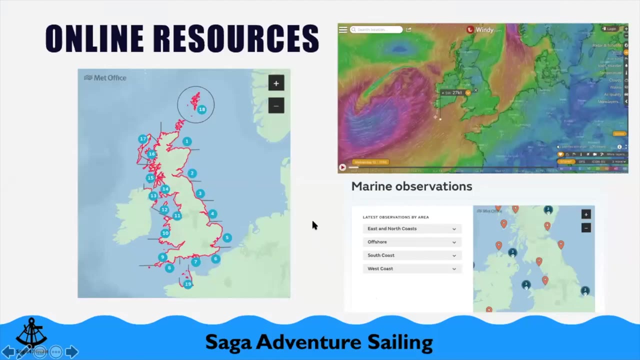 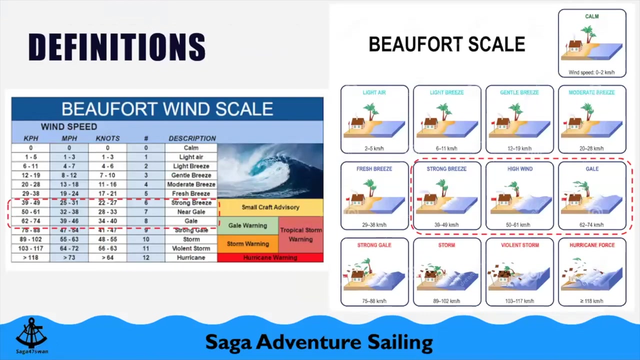 how that apps is working for your local area. Okay, so let me just get back to my presentation. Okay, All right. All right. So definitions: We talked many times about F6. And F9. So they all referring to something called the before. 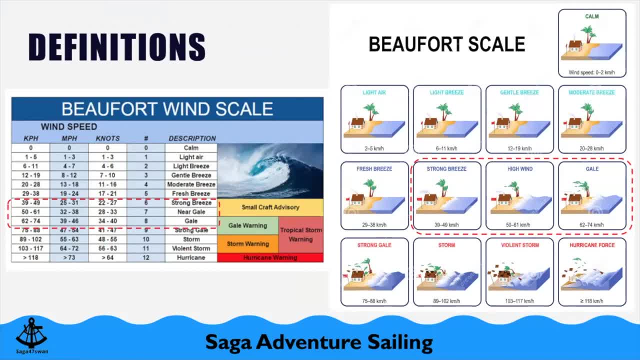 scale. the wind scale, which was made many, many years ago in a time of Lord Lord Nelson, was an admiral. before he made a wind scale so that so the young officer could find out when to take the sails down, When, when you are sailing and the wind is. 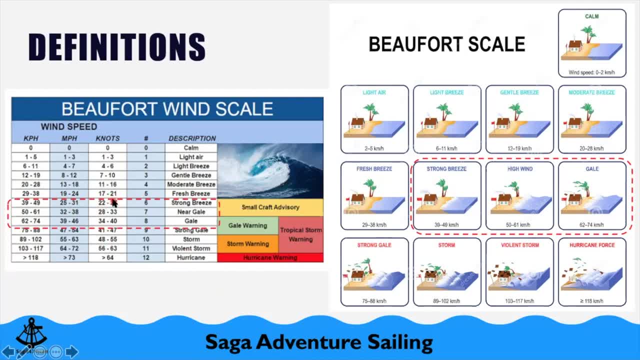 starting to get up to what Call around for six, for seven and for eight. That's, it starts to get quite windy And if you are not out there, then when we get to these kind of wind forecast, then you should consider if you really 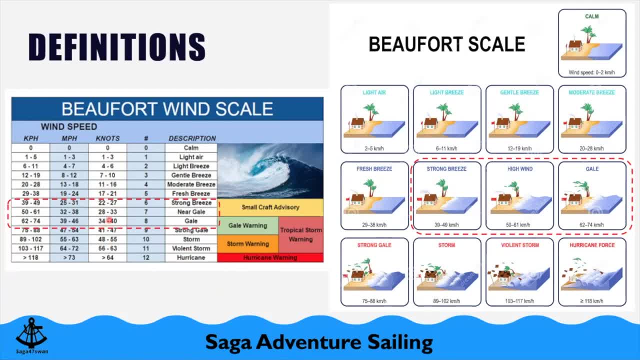 need to go out there, Because if you're- especially if you're- beating into the wind, it's not going to be very much fun to be in for six and for seven. Yeah, I have a drawing here on the other side where you can see that when we get to, these kind of winds is 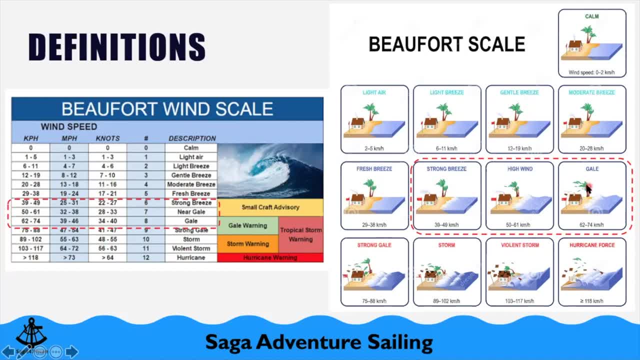 when the, the roofs start flying off the houses. So it's quite, quite windy. So the inshore weather forecast will turn red for six and the and the shipping forecast, the offshore forecast, will turn red at the gale force force eight. I mentioned before seas that it's so. 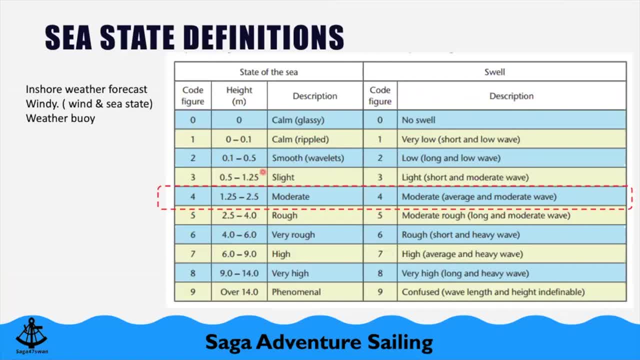 so important that you check the sea state here, because that's what's going to make the sailing uncomfortable, Yeah, And you also have to take into account. so we have moderate, moderate here. So I take it a lot of people have been out sailing in moderate sea, which is two, and 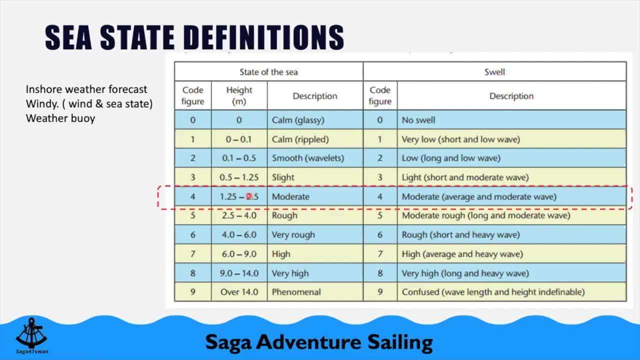 a half meters away And they definitely said: Oh, this is, this feels quite rough. Yeah, And it does. And also because these sea definitions are actually made for big supertankers. So moderate is okay for supertanker, but for small vessel it starts to feel a. 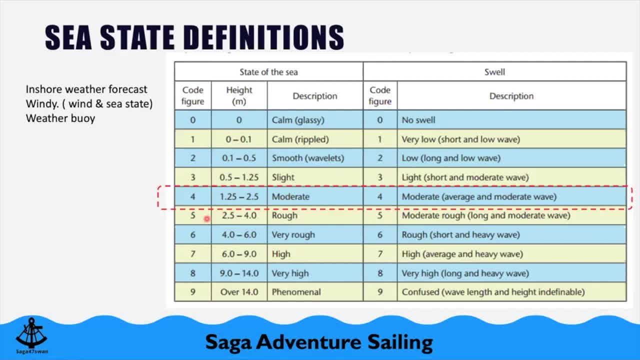 bit rough, Yeah, And when we get up to rough seas, which is waves up to two but from 2.5 to four meters, it starts to get danger. can get that dangerous because when they say that if the waves are the height, 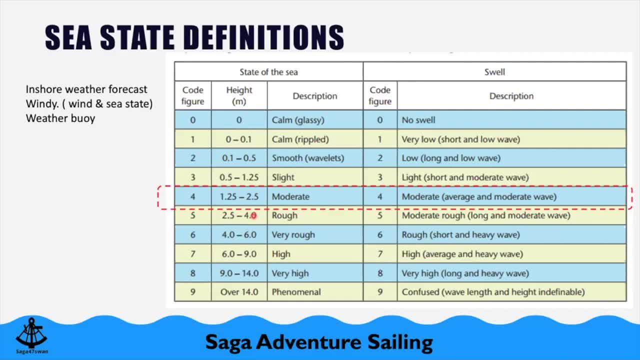 of the waves are the equal to the width of the boat, then they can breaking wave can can roll over the boat. Yeah, So you have to be really, really careful when you start to get in that kind of seas. Okay, other definitions that we have in the fellow podcast is: 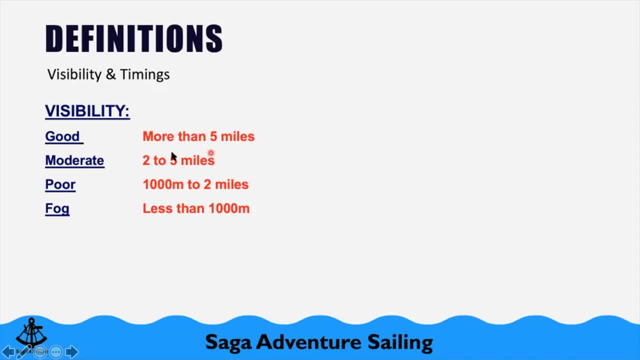 visibility. So it's visibility is how far we can see. So good visibility is for more than five miles, moderate two to five miles. when it starts to get down to poor, Then we had to start thinking about if we need to go out. 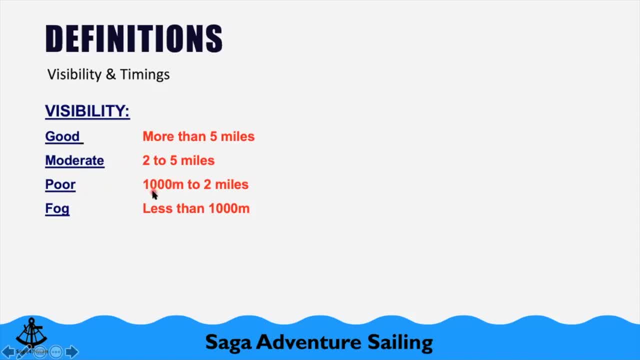 because it's not a very good idea to go out in the shipping lane and English Channel or in the in the solar because there's so many big ships. So then you stay in the shallow or you wait in port until the the fog clears. I mentioned also earlier about gale warnings and 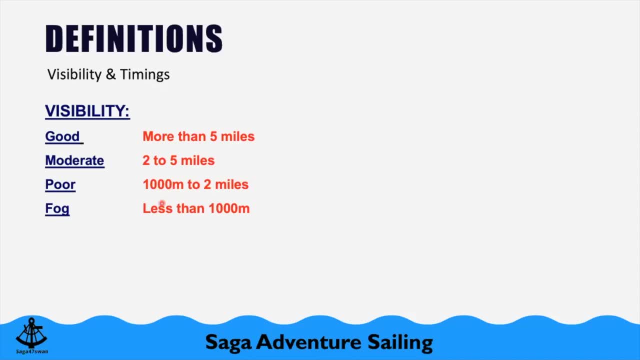 timing. So you have to be very careful when you're going out in the English Channel, especially if you are in an area with, like the Solent and it's fucking conditions as a sea fog there, then it's not a very good idea to go out in the shipping. 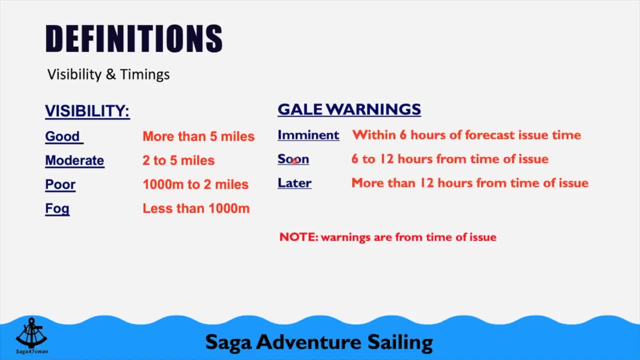 lane And with that you have to have a weather forecast. So you have to have a weather forecast, So you have to have a weather forecast. So again, when you have a weather forecast and assess that gale warning is expected soon, that means from six to 12 hours from. 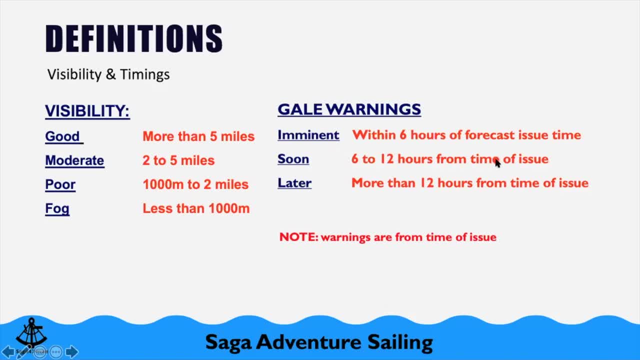 the time of issue of the weather forecast. So if the weather forecast is eight to 10 hours old when you listen to it, then gale is just around the corner. So that's very important that when you are listening to a weather forecast, that you 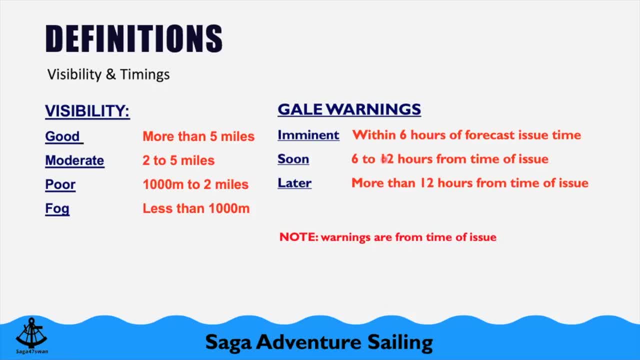 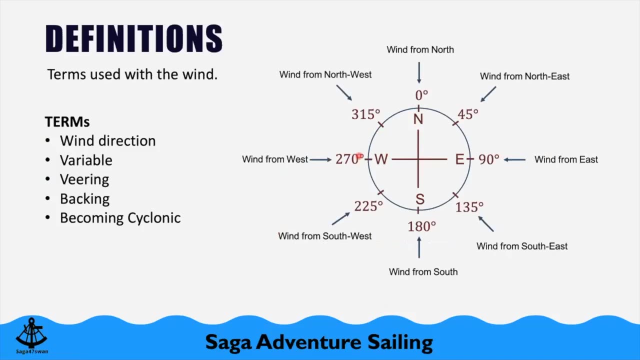 understand When you hear the weather forecast. you are hearing a lot of that weather forecast is issued for. they will clearly mention that in the beginning of the weather forecast. it's very, very important. all right definitions for wind. so for the wind, we have the wind direction. the wind direction is: 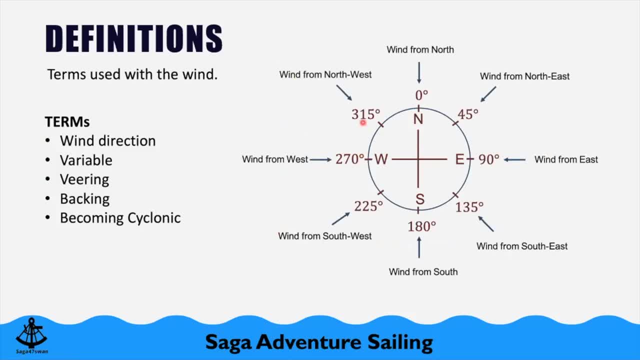 if the wind is from northwest, that means it's coming from the northwest. if there was also sometimes mentioned that the uh, the wind is variable and that means that the wind is coming from all over the place. we find that many times when a um, when the anti-soclone, that 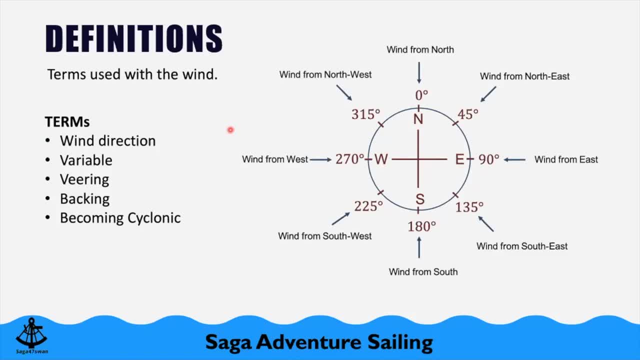 means the pressure system is just, uh, on top of us, passing over us. we also have a saying, a word saying: wearing that the wind is wearing. that means the wind is turning and the wind is moving and it's turning clockwise. so if the wind was west and it's wearing, it will wear towards. 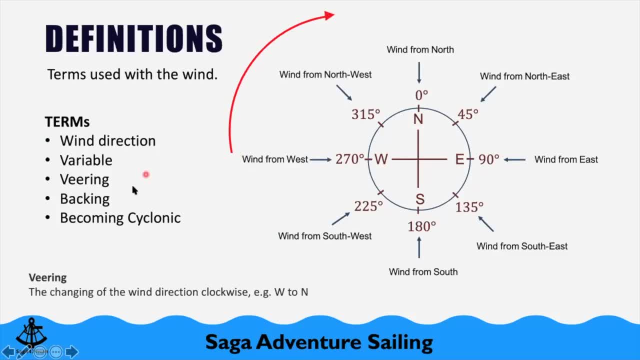 maybe, for example, north back in. that is easy to remember. uh, backing is like going against something, so anti-clockwise. so if the wind was east, it would be back and going up to north, for example. the last thing we have is cyclonic. cyclonic is when the depression 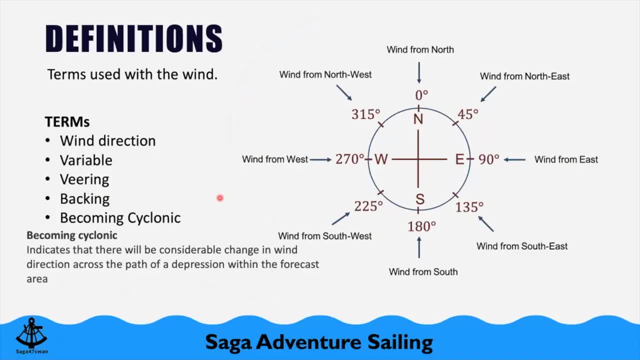 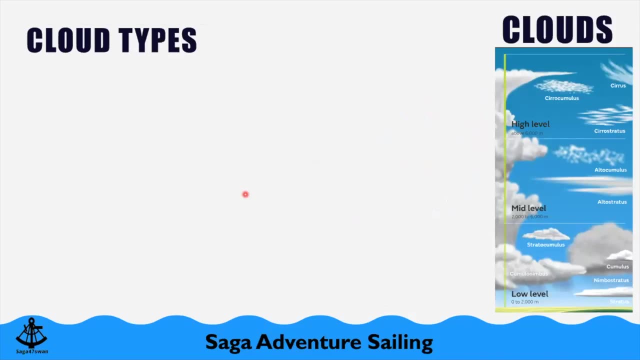 and the wind system is passing us either to the north or to the south of us on its way in the eastern direction, then the wind will change as the wind, as the depression is passing us. Clouds- Okay, there's so many clouds and so many definitions of clouds there, so it can be quite. 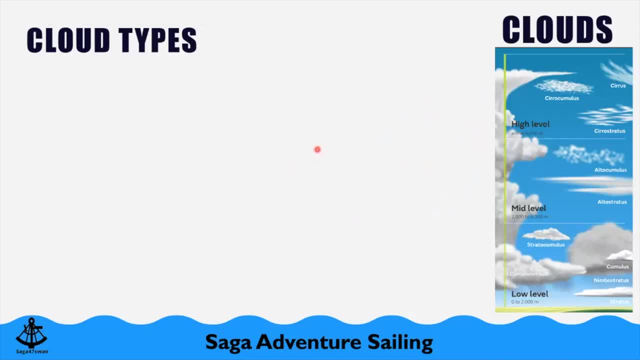 mind-blowing to try to figure out that- all these clouds, But we actually only need to remember about six terms. So then, with these six terms, we can build up the majority of the clouds. So there are three main types. So we have Coulomus clouds. They are like heap or lumpy. 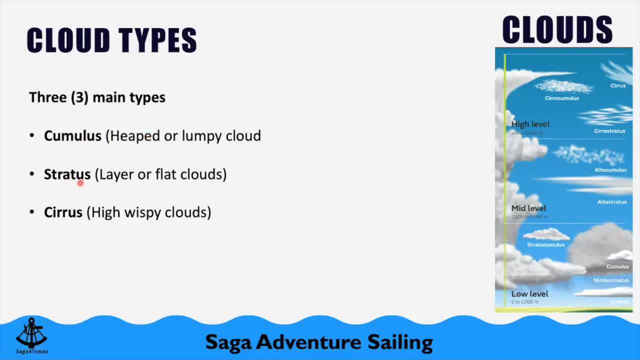 fluffy clouds, Stratus clouds. Stratus means layer or flat clouds. So we have example here, Altostratus here. And then the last type, the third type, is Sirius. They are means high whispering clouds. So they are the ones which are up here. They're mainly 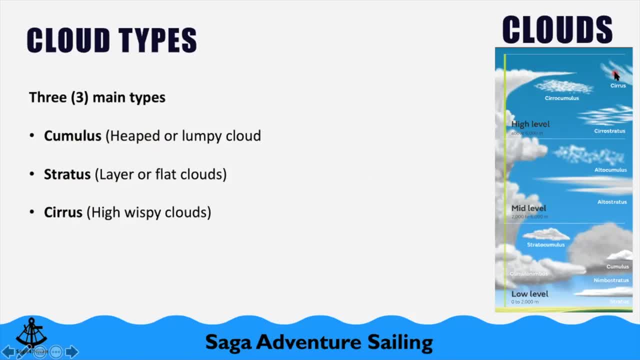 ice crystals, Very, very fine clouds. The next thing we have to add to that, to the characteristics, is something with the height, So high levels, Sirius. So we have like, for example, up here we have the Sirius Coulomus clouds- So high fluffy clouds up here, Also sometimes called Macral sky. 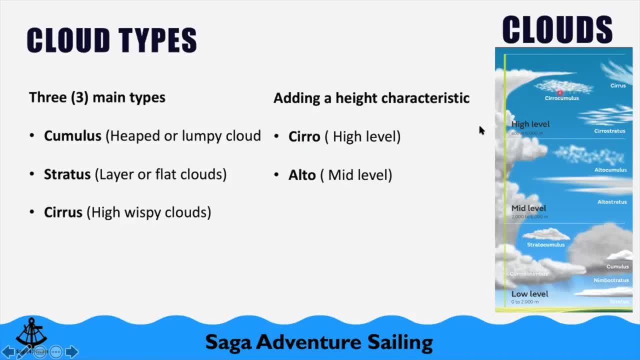 because they look like the fish scale on a Macral. Or we have like Alto, So we have like Altostratus here. So mid-level layer cloud is there, And then the last thing we need to add to that is we need to know if it's dry or rain bearing. 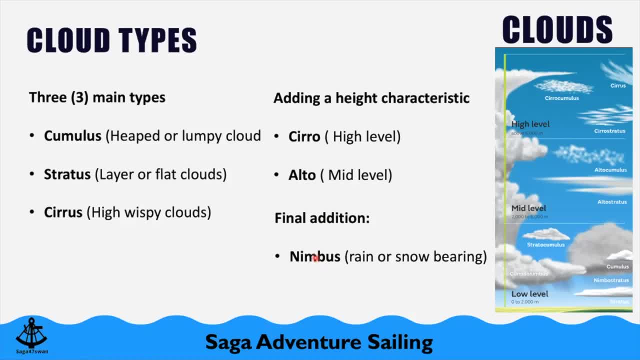 So we add Nimbus to it. So if a cloud has rain or snow in it, we say it's, we add Nimbus. So, for example, here we have Coulomus Nimbus, So that is a fluffy rain bearing cloud, Or Nimbus stratus would be a layer cloud which is rain bearing, If you can remember those six. 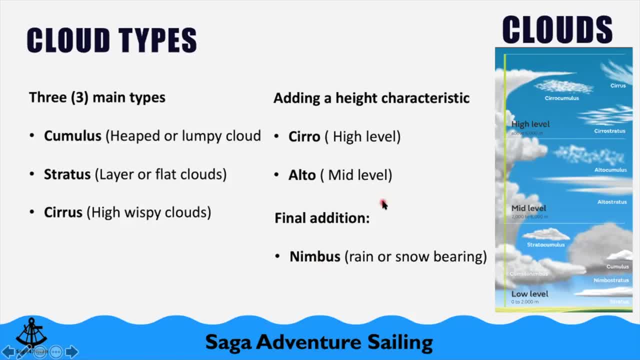 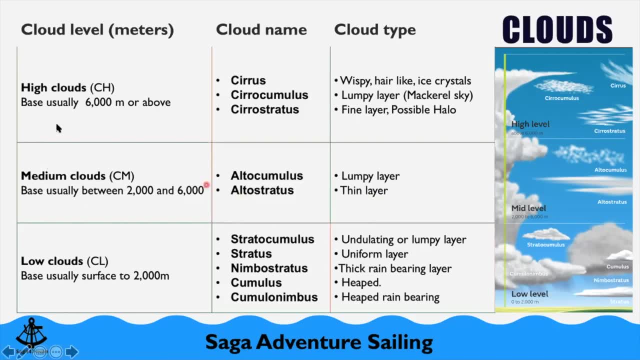 terms, then you can build all the clouds accordingly. So this is all the clouds, basically. Again, so we have the high clouds, Sirius clouds, medium clouds- Both are mentioning Alto- And then we have the low clouds And the. we can add Nimbus if it's rain bearing, Or stratus if it's a layer cloud. 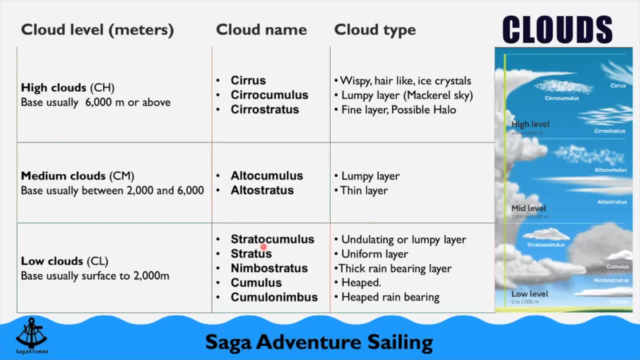 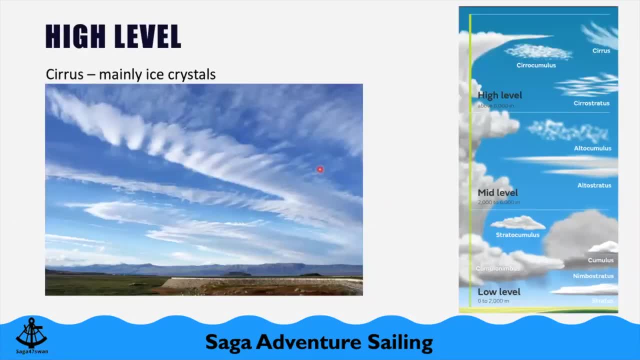 I'll just go through the. I'll just show you all the all the clouds now one by one. Just quick go through them. So we start at the high level. We have the Sirius Coulomus, So this is the Sirius cloud Up in the top- again mainly ice crystals, very, very fine. 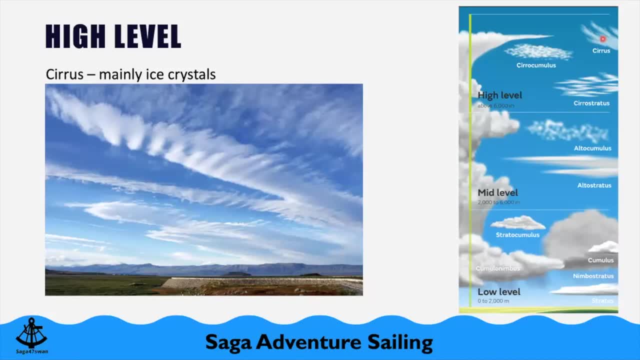 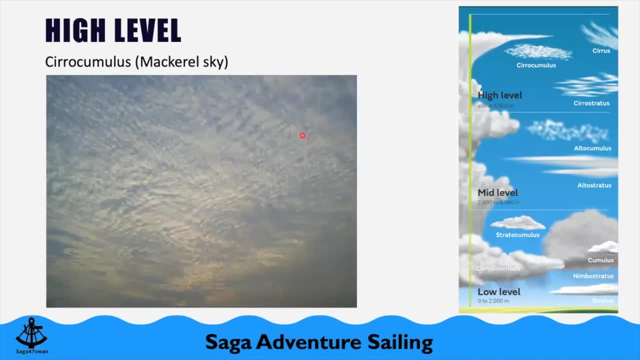 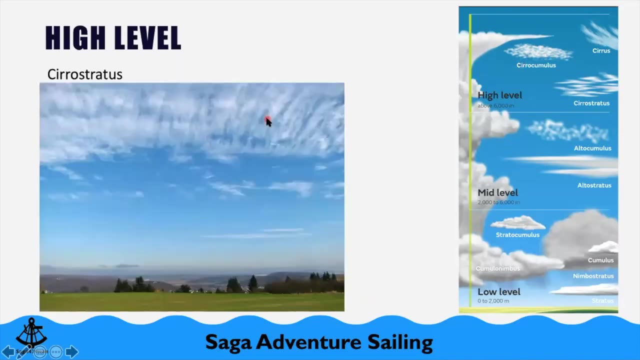 Normally associated with a nice weather, sunny. Then the next one we go down from there is the Sirius Coulomus cloud, also called the Mackerel sky, like here, And then the next one will be the Sirius stratus- Fine clouds, again high, But a layer cloud. 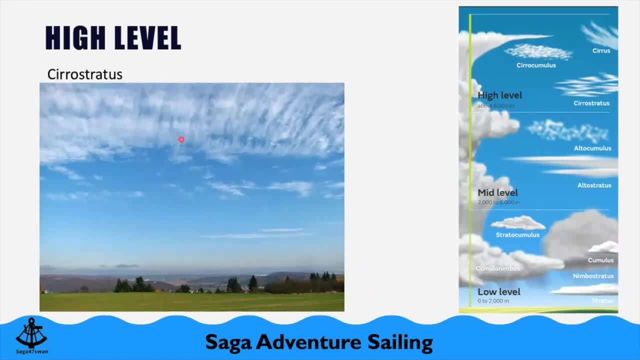 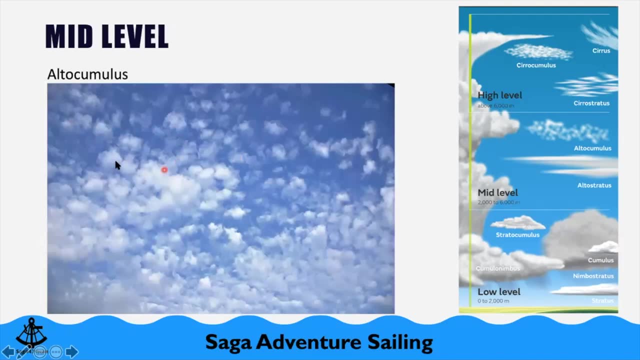 Then we move one level down where we get the mid-level clouds which we again have here. So Coulomus, we can see it's fluffy and it's sort of a layer. So this is Alto. Sorry, not sorry. 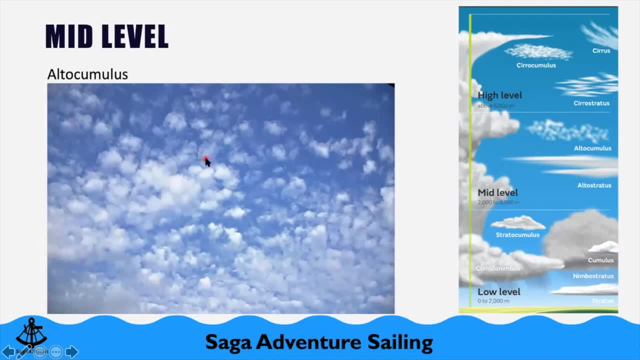 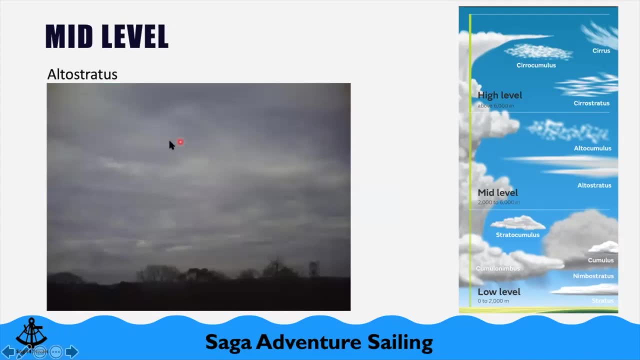 Alto Coulomus is fluffy clouds at the mid-level, And then the next one would be the layer cloud. So then here we have the Alto stratus. You can clearly see typical British clouds. yeah, Dark 4. You can also see known 서울 clouds from the sub-seasilging signal f trên the layer clouds. 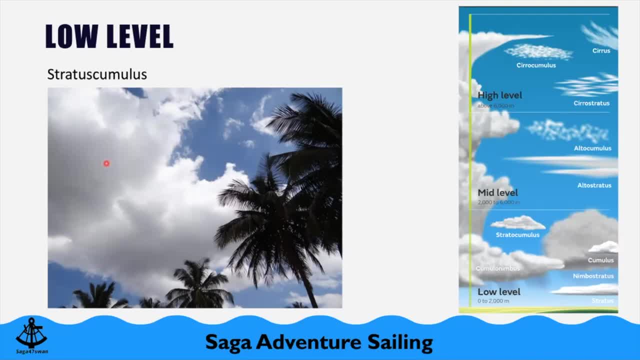 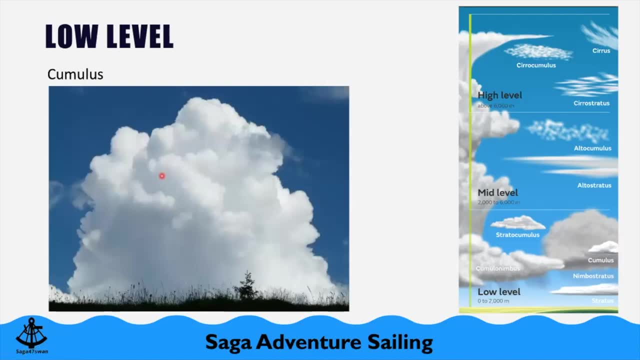 And then we have the stratus coulomus, which is again a layer cloud which is fluffy. Oh, I have some palm trees there. It must be down in Cornwall. And then we have Coulomus, so Coulomus clouds Again, when something is fluffy and it's building up. 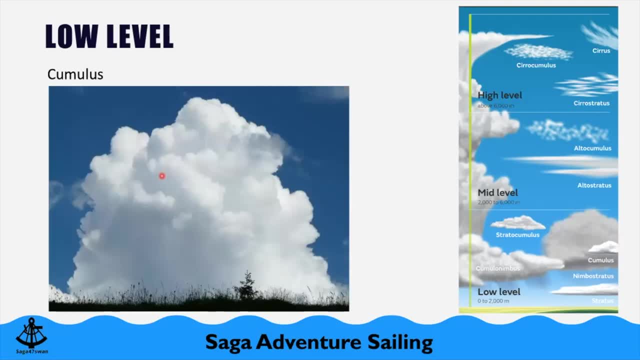 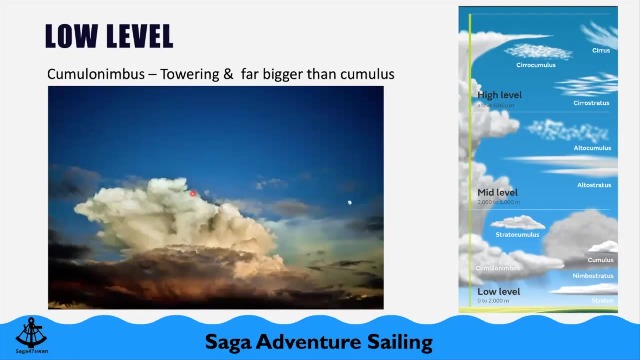 it's indicating that we have in the, in the, in the weather system is moving up, air is moving up, we'll get some, some wind and so on, and then we get to the culuvus nimbus- again very instable, unstable clouds, powerful building up, towering up and they will create a wind and and rain, and then we have the nimble stratus again. 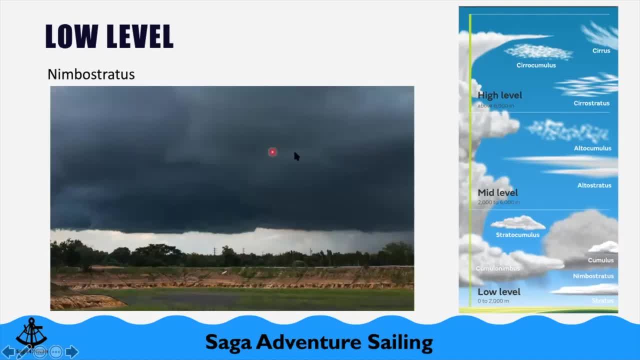 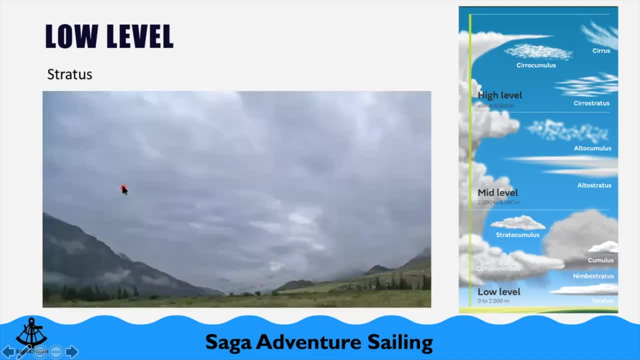 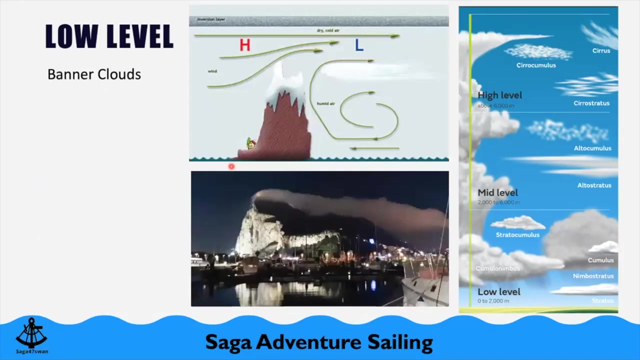 layer, stratus is layer, and then nimbus is rain. so here rain bearing or snow bearing clouds, and again normal stratus clouds again. so those are the, the cloud levels, the cloud types. i have one more cloud which i think is very, very interesting. it's called the banner cloud. banner cloud is associated also with 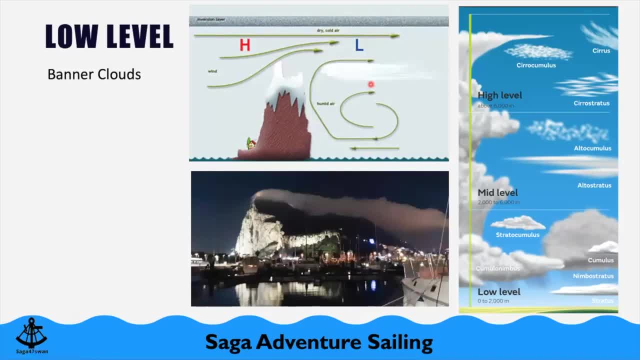 making landfall. so when, in the old days or also now, when you're sailing in the open seas and you are approaching land or an island, then the first thing that you will see is a cloud hanging over the over the island, and i have a picture here. it's not the best picture, it's a picture i took. 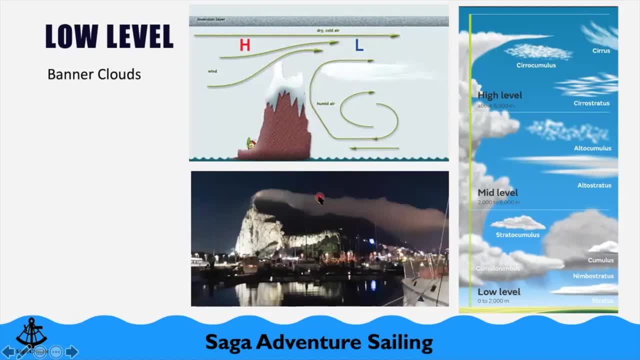 on our sail back from italy last year during covid. this is a rock of gibraltar and then you have the, the layer cloud here, so it's beautiful lying there. so that's a picture, that's a first thing you would see when you, before you make a landfall, you would see the. 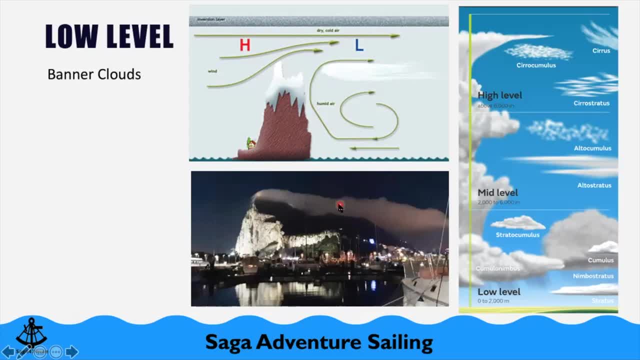 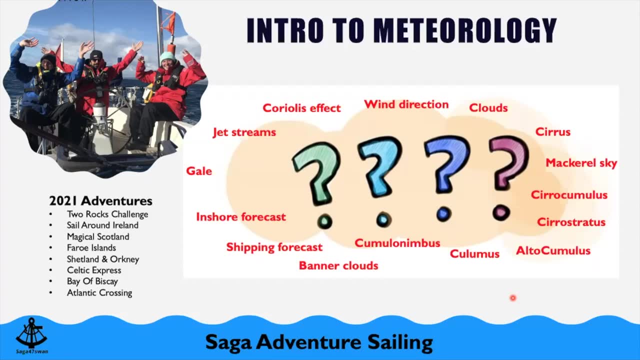 you'll see the clouds, the banner cloud. joe has a question and i think you can relate to that. so he said i have heard the bay of biscay is very challenging sailing. is that because of the weather? why is that okay? so the bay of biscay is um, it's a uh, why it has such a bad. 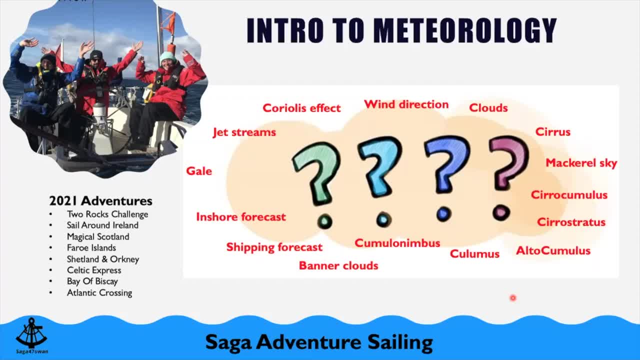 reputation is in the old days the ship they did not beat, they did not sail very well close to the wind. so if there was a storm- and the storm, the wind will mainly come from the west or the northwest or southwest- and they got into the bay of biscay. they could not get out, so they will be put on the 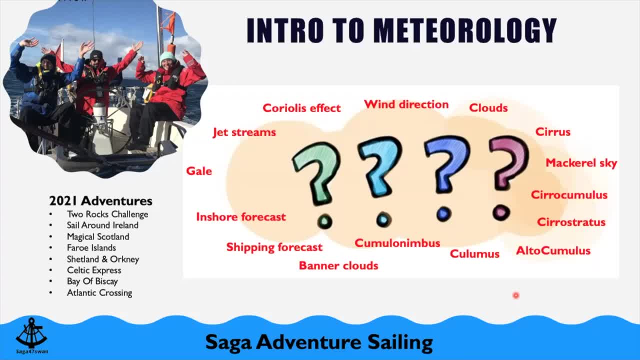 rocks, so that's why it has such a bad name. second thing which is affecting the the bay of biscay is the sea state there is very, very bad. the reason is that the atlantic is several, several kilometers deep, but when we get to the biscay then suddenly it jumps from several kilometers to very shallow. 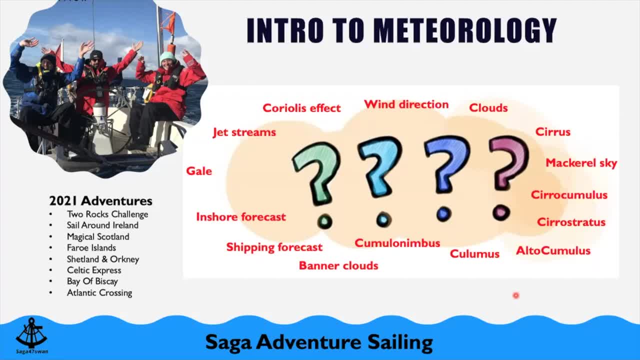 about, i think, 60 meters, and that's why you get from uh, from the tip of um of uh, spain, north portugal, spain, up to uh, up to france, uh, you get washing machine area uh in there, so there could be very, very confused seas there, where that. 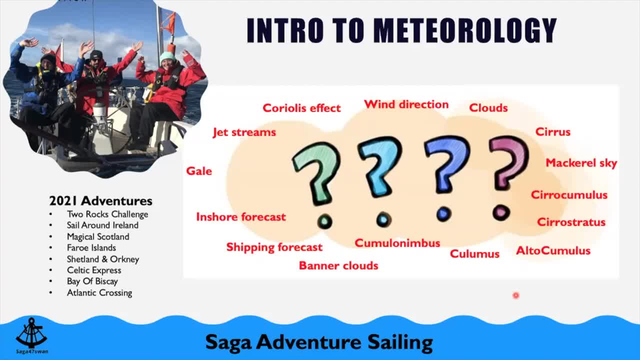 that happens. so, uh, there are three ways that you can uh cross the bay of biscay. you can go offshore, so that means you go to the lands end and then you bypass that bad area, or you take the, if you have time, then you go along the coast all the way around and stop in all the ports and 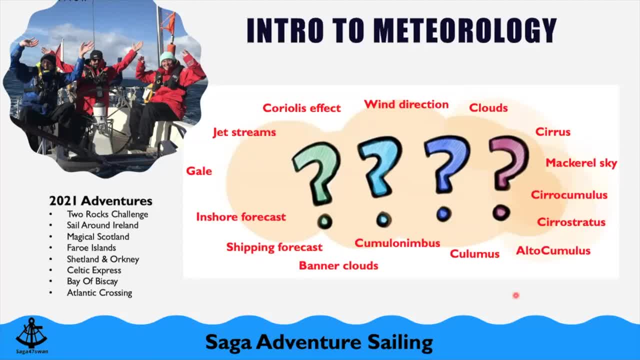 have lots of uh, wool and shrimps and all these things, or you wait until you get a very good weather forecast, and now the weather forecasts are very good. so you need a good weather forecast for for three to four days and then you uh shoot across, uh in the in the direct line, like uh, like natalie and i did, we waited there in.